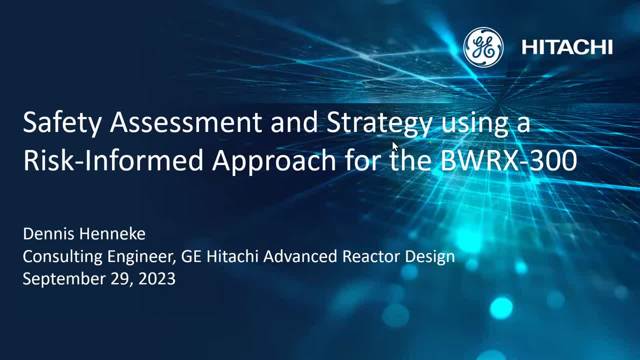 Please welcome, Dennis. The floor is yours. Thanks, Ken. I see your names on there. old friends At least know half of you, so that's good. And, like Pat said, if you have a short question, clarification or whatever, this is a question. 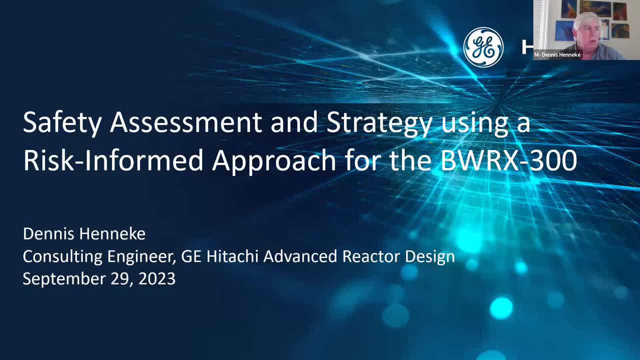 So jump in. Jump in during the call at any time, But if you have longer questions we'll wait until the end. I'm the kind of senior person for GEH Hitachi for both BWRX-300 and Natrium. 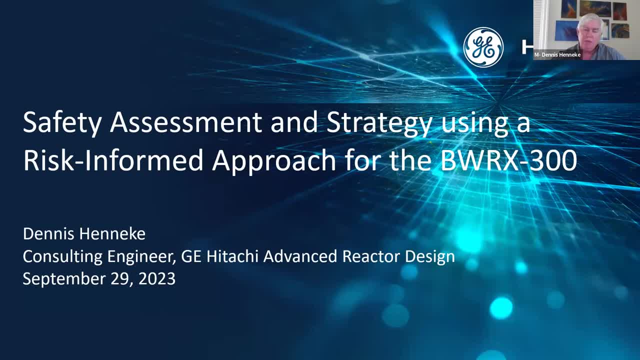 I am on the technical side of GEH And we have a lot of people- a number of them- on this call. I think we have them. I'm going to be presenting their work. I'm sure all of them will be very proud to talk up and present their work about the X-300. 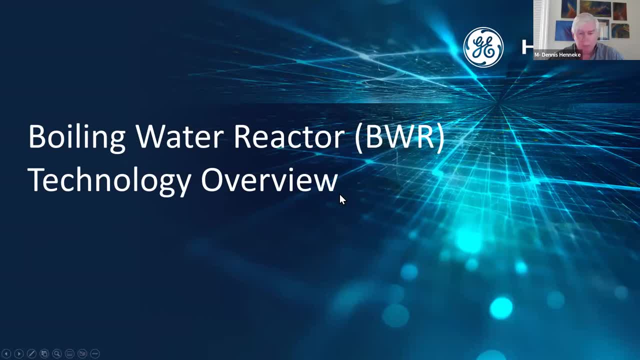 So let me go through a little bit just on the X-300 first, and then get into the risk-informed approach, Talk a little bit about the IEA approach- Some of you may have heard me talk about it, We've talked about this in other venues- and then talk about the safety strategy that we're utilizing for both the Darlington site in Canada for the X-300, as well as the TVA site in the US, with some adjustments to meet the US requirements. 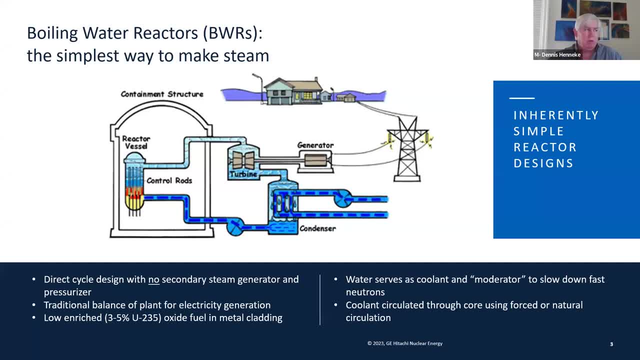 So BWRX-300 is first and foremost a boiling water reactor. So those of you who aren't familiar with the boiling water reactor, it's a lower-pressure reactor than a pressurized water reactor, because the steam that's produced in the reactor vessel here goes directly to the turbine generator to produce electric power, to feed water and condensate. 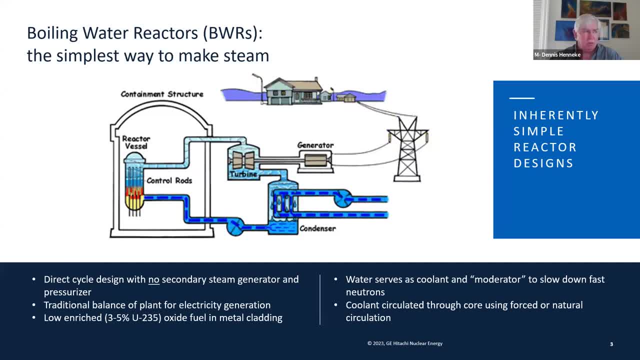 Much simpler design than a pressurized water reactor, And there's pluses and minuses. I was a PWR, a PRA engineer. I was a PRA engineer for some 24 years as well as did some startup work for Palo Verde and Sharon Harris. 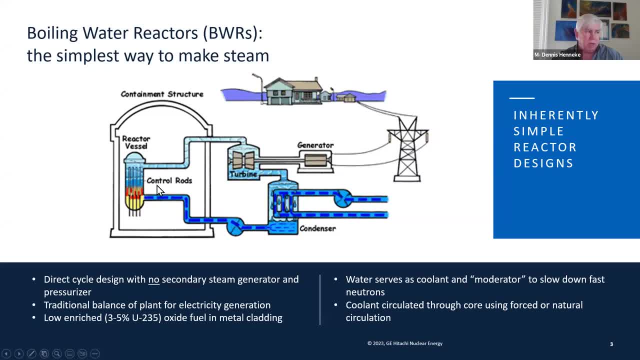 So I see pluses and minuses in both. The simpler design does help us in the area of SM and advanced reactors and you'll see here in a little bit why that. And of course you have a radioactivity- slightly radioactive- steam turbine generator, so you do have to shield that and you have to worry about that during maintenance activities. 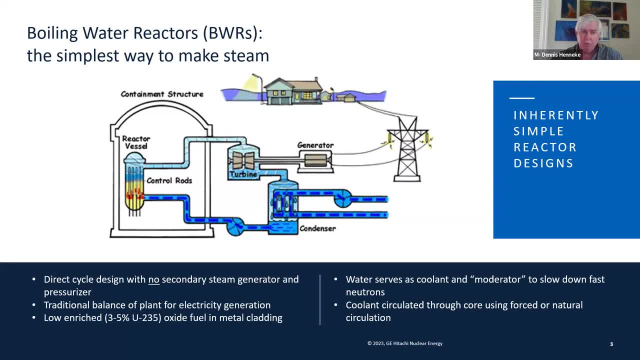 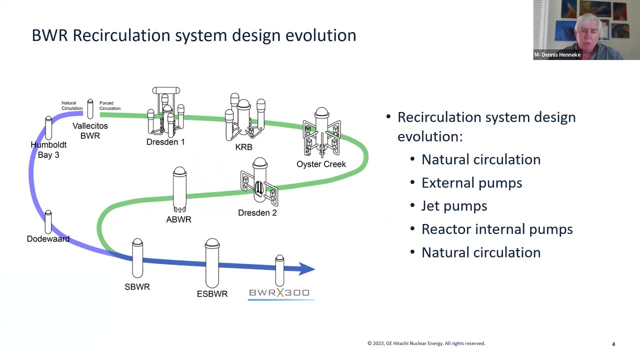 But otherwise the simpler design does allow us to get a plant that is brisk and simpler than an advanced PWR. As far as historical from a GE standpoint, we actually have two different routes to get where we are today. You'll see the very first reactor that was licensed in the US. 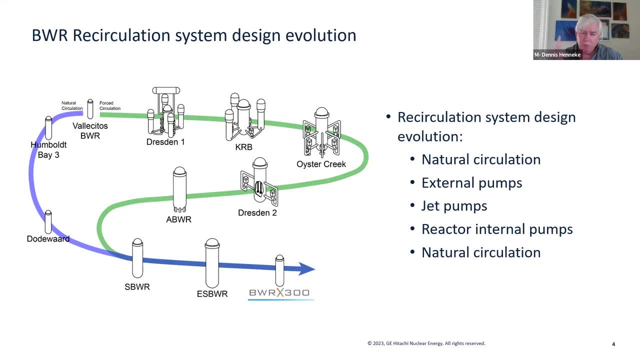 is the PWA That was licensed number one in the US for plants That was a natural circulation plant And built several reactors that continue to be natural circulation plants, Humboldt Bay- and I'm sure Mr Budnitz has some historical reasons why Humboldt Bay was probably not successful- 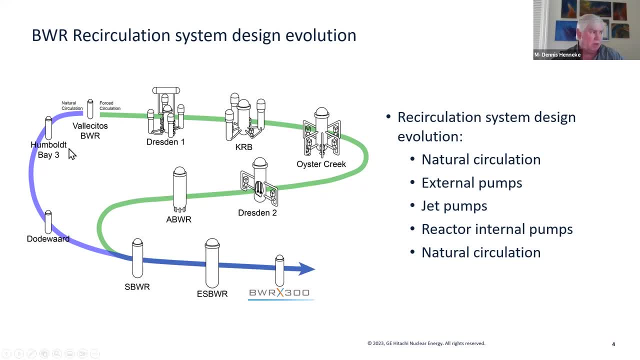 Built probably in the wrong location, near seismic activity. But there were others. There were other issues with regard to that plant and then Dodewaert, over in the Netherlands, plants that continue to be natural cirque But as we try to increase power, the designers felt that forced circulation was needed. 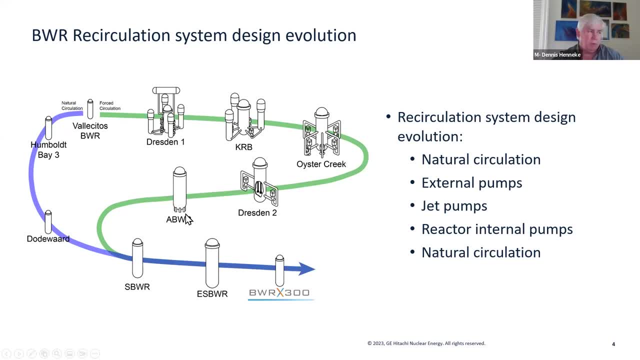 They went to the PWR 1,, 2,, 3,, 4, all the way through the advanced boiling water reactor, which has still forced circulation, but in reactor internal pumps, Eventually coming back to our design for the EWR. 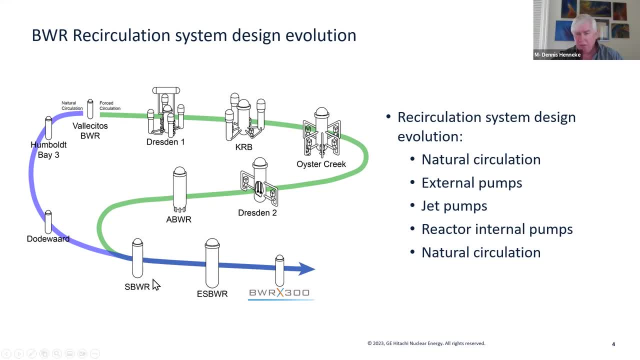 the ESBWR, which was fed from the simplified boiling water reactor ESBWR, we got back to natural circulation in the 1900s And if you count that, there there's of reactors And that's the X-ray. 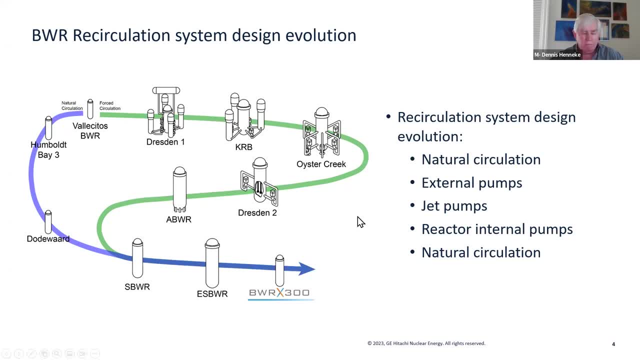 Our attention to the reactor So for a long time felt like natural circulation circle is the way to go, and it's especially true for a smaller reactor. but we went away from the operating fleet. They have a circulation with external circuits. 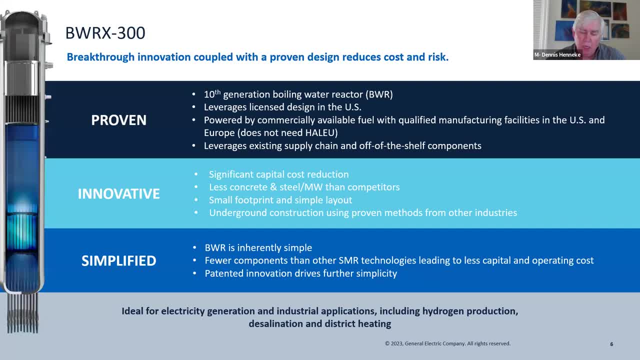 As far as the BWRX-300, it has some first-of-a-kind attributes, but one of the things you'll see on the next couple of slides is we are trying to use proven technology. We're using existing fuel, existing internals, existing control rods, existing technology. 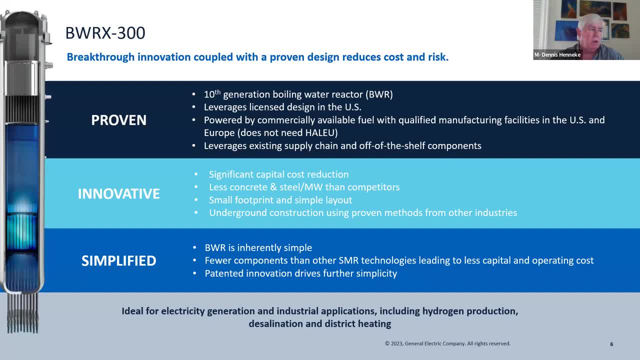 in almost everything we do, with a few exceptions we'll go into. If you were to try, for example, to develop an advanced reactor where you had a new type of fuel and you had to go through licensing for that fuel, that does add years to your 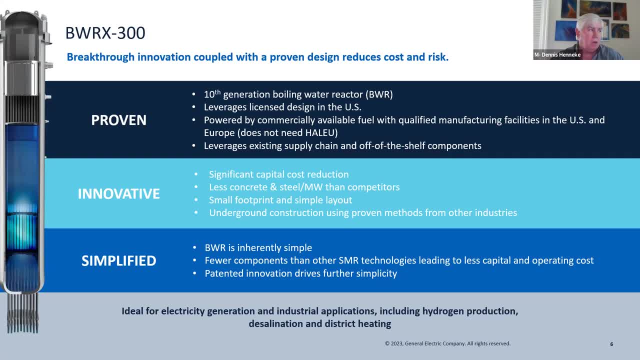 license, And so we're using the same fuel as the existing fleet. That does help us. On the other hand, we're using innovation where it makes sense from both a risk standpoint and a cost standpoint, And I'll talk a little bit about a few of those. although the design of the containment 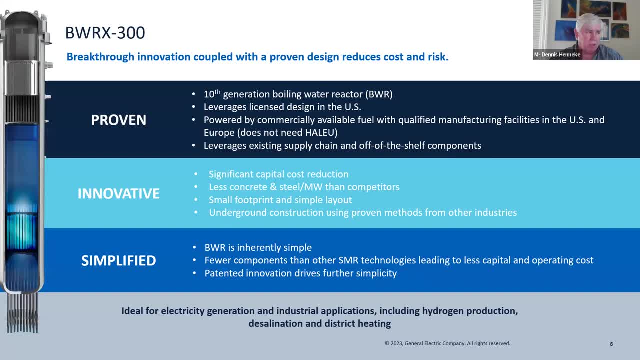 and the steel composite structure I'm not going to get into. Mainly the thing about the X-300 is it's simplified over previous designs, even over the ESP, And this results in about a total about 20% of a typical boiling water reactor and 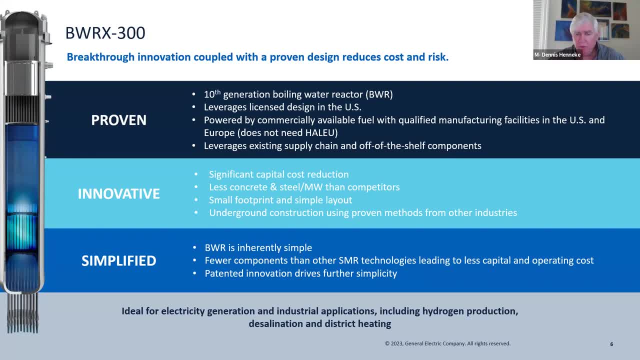 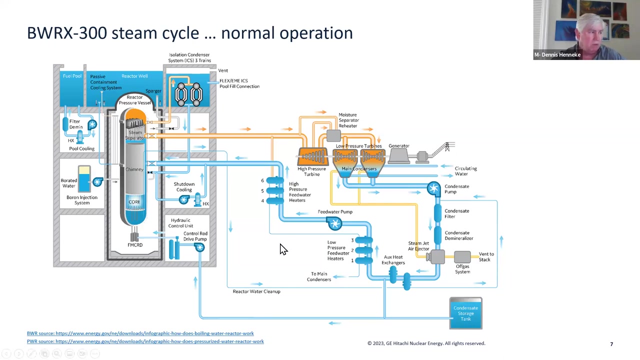 less. we'll call it safety foot- smaller amount of components we have to protect from, say, a seismic standpoint or high winds, and so less capital costs, less operating costs overall. This is a layout of the BWRX-300 with most of the major components shown. 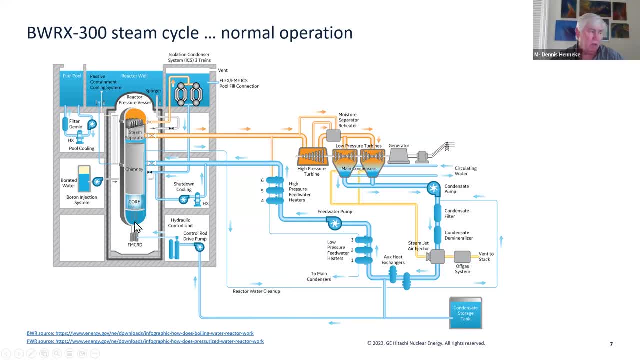 The reactor here is large, most in order to natural as well as reduce over moisture carryover into the turbine generator to help minimize the amount of radioactive steam that might be produced. And it's going to be a nice, nice solution on a planned project, if, of course, we're. 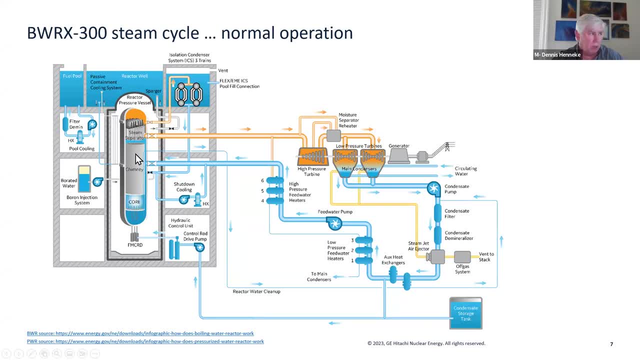 building something that's going to be built so that it doesn't hit a water pipe, Then I'll grab on to it right away And it's going to be a little bit more sophisticated here, with a lot of more modern equipment, And we'll make sure that it's going to be used consistently. 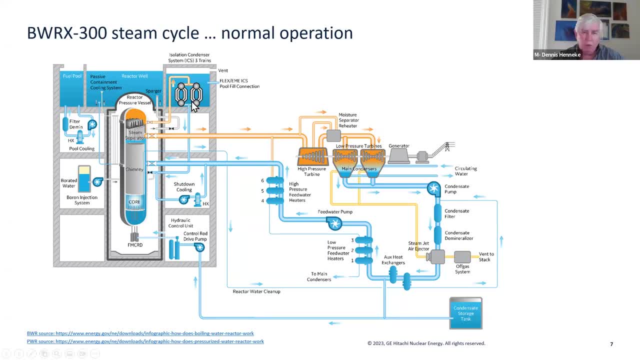 Everything else here, with regard to the control drive system or injection, everything else here is similar to previous plants. One key is the isolation condensers and we'll get into that here in a minute. but if you From a passive standpoint, it's a passive cooling system. 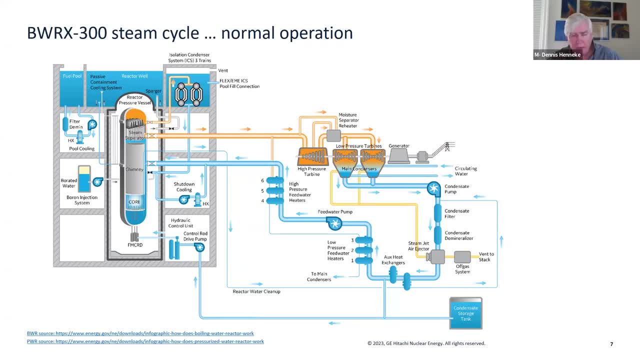 If you can make that isolation condenser very reliable, which we have, that's a key to the overall safety of the plant. Change the design of the isolation. I'll get into that in a minute, But other than that, this is a simplified version. 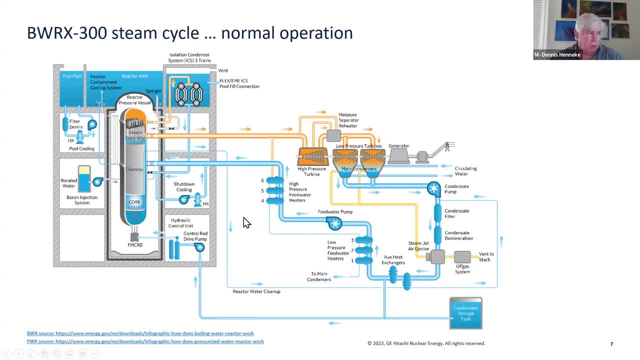 including the secondary side of a boiling water reactor. The other thing is, because it's a 300 megawatt plant and relatively small, we're able to build a much smaller containment And, if you'll notice, this is a first in a long time. 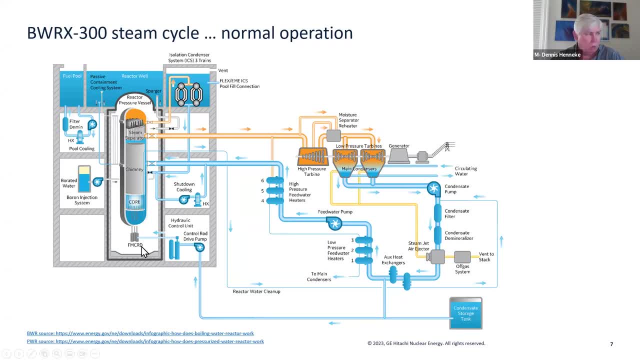 that we have a boiling water reactor. It does not have a suppression pool, And the reason for that I'll get into in a minute. but that mainly is that the isolation condenser not only supports decay heat removal but it also supports pressure control in the primary. 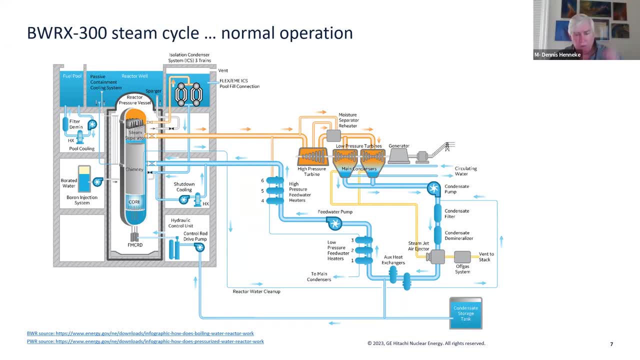 So we don't have. So we don't have a need to open relief valves or pours down to a suppression pool in order to A design basis event or even beyond design basis event. So no suppression pool reduces overall containment size. It does add the need which you'll see up here on the upper left side. 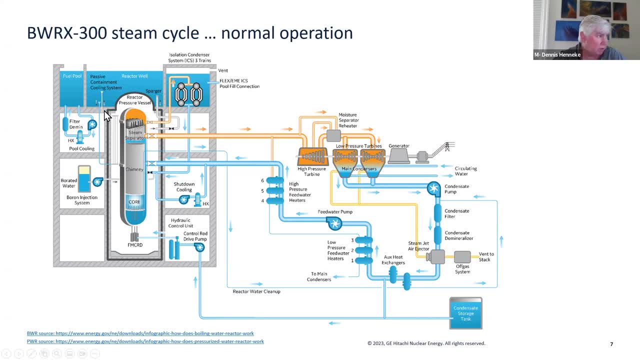 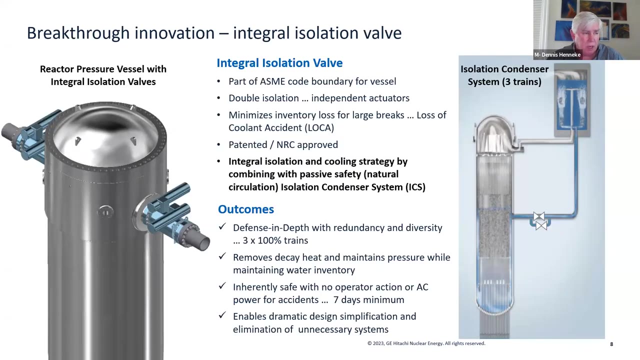 the need for a containment vent. Sorry, it's coming up through here. So we do have a containment vent or containment overpressure protection. that's needed for the design Part of the reactor design that's important- are these isolation valves Now normally in previous design? 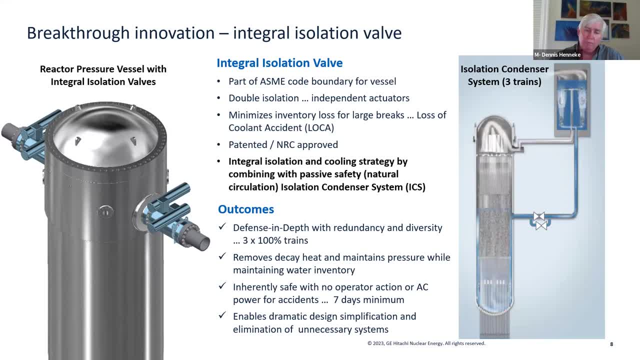 isolation valves were containment isolation. They were on the containment boundary. We've moved them in all cases next to the vessel, So there really is very little room between the first valve and the vessel itself And what we're able to do is move a large, medium loca event. 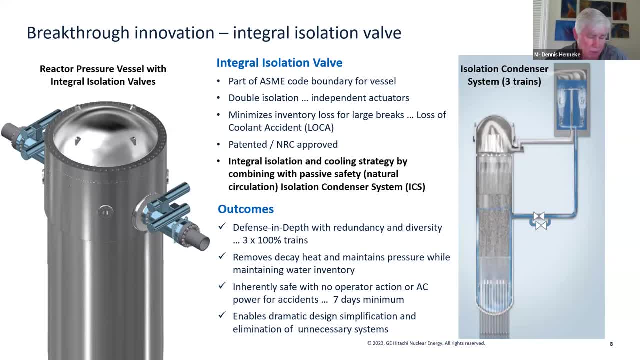 to the design basis space. But once the valve closes and can isolate, then pretty much most locas are stopped from impacting the safety functions, And so that helps us in overall safety. So these interval valves, one beside each other, they're still being designed and they do help us. 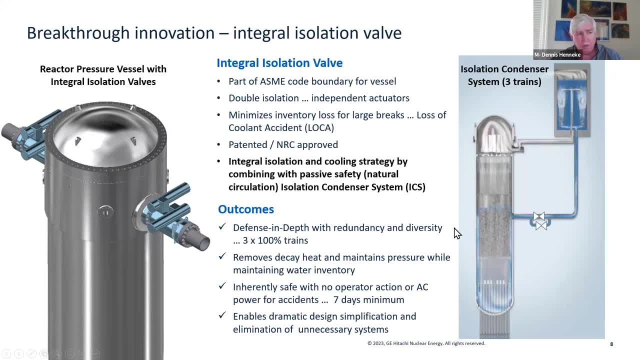 We isolate the primary entirely and you'll see over on the right here now. this is one of the isolation that open up and then to a large And you can operate these without any operator action in the case of isolation. You'll also notice two valves here on the return line. 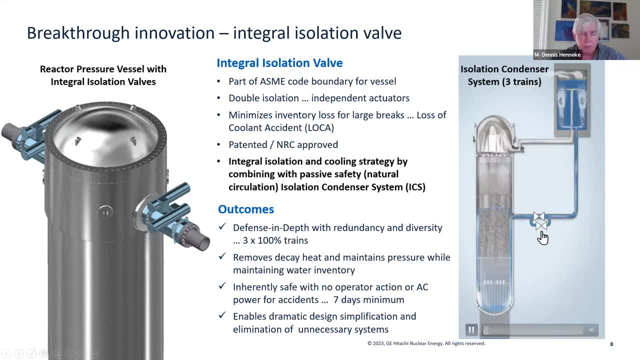 Those are normally closed. This is the reliability improvement we have over the year. And those the valves. one is a safety relay valve, one is a non-safety relay valve. Either of them opening- they both feel safe- will result in isolation denser being opened. 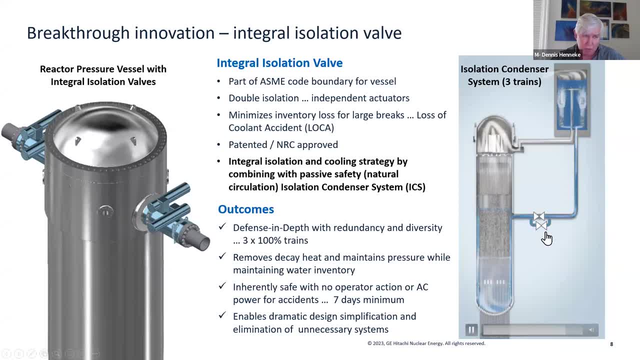 So we were able to take what was the pinch point for the reliability for isolation densers which a lot of you have heard me talk about- software common cause, driven by software common cause and digital INC, which was about a 10 to minus 4 failure rate. 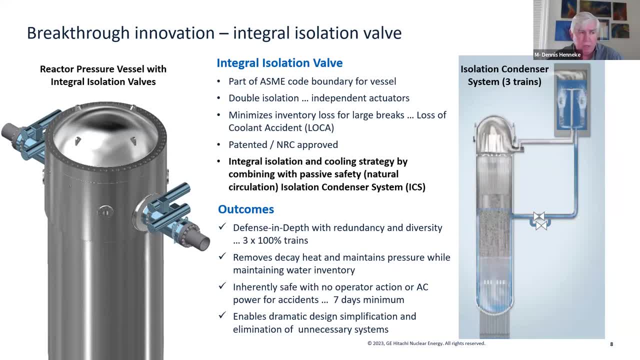 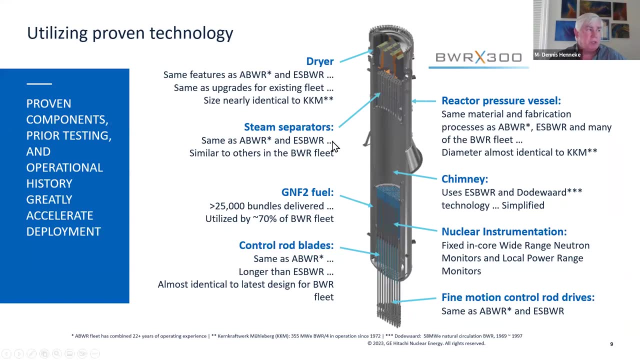 And now we're able to reduce that down to something in the order of 10 to minus 7 failure rate for isolation densers. So we have a much more reliable passive system here with the current isolation denser system, The vessel- So I think I mentioned most of this- is all proven technology. 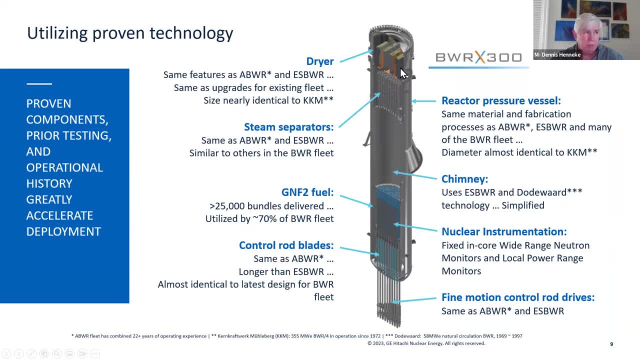 the same fuel, G and F2 fuel. same steam separator: reviews before. same steam dryer. a similar reactor vessel, although a little bit longer and skinnier than our previous designs for the ABWR and ESPWR. It's very similar to the KKM site, and so on. 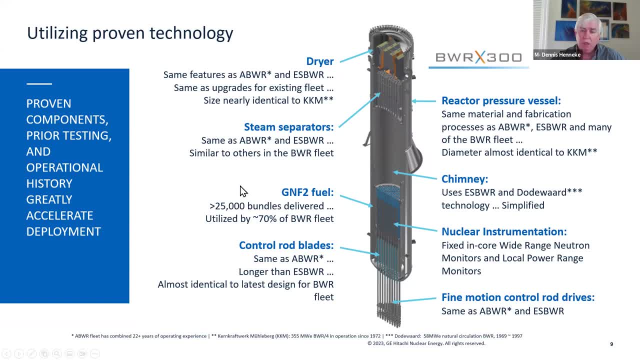 So we're not trying to design this with anything new. Yeah, So basically, inside the vessel, the isolation denser is, although we've used isolation densers and other plants such as DOTAWAR. we had it in the ESPWR. the operating fleet had isolation densers in the BWR1, but not since then. 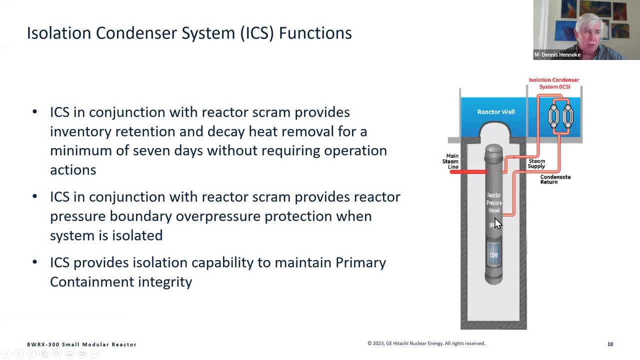 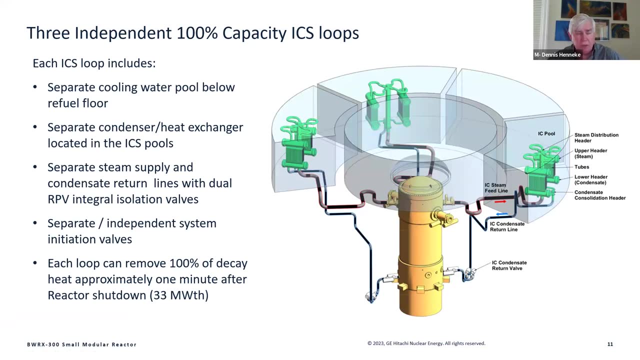 And here's a simplified diagram of that isolation condenser system. I think I've covered all of this here. Here's a little more complicated diagram. You can see the isolation condensers are actually two sets of heat exchangers, or two heat exchangers per train, three trains each, each 100% for a typical reactor trip. 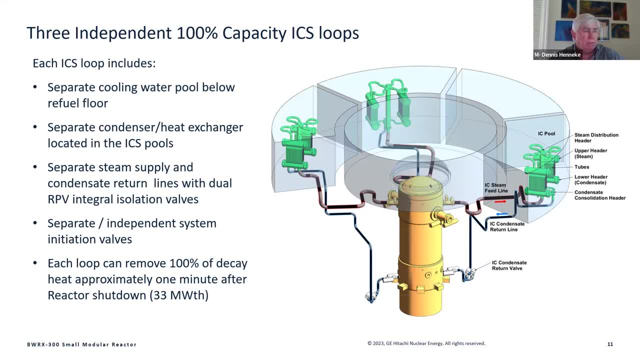 33 megawatt thermo can be removed from the reactor. And then you can see here the return valves, the two valves, two valves here. So all we have to do is open one of the three trains in order to get cooling, for a typical event. 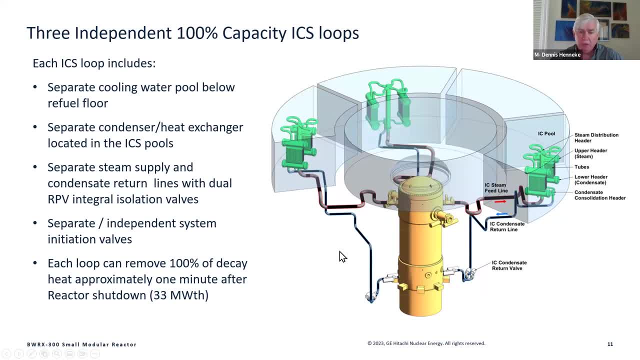 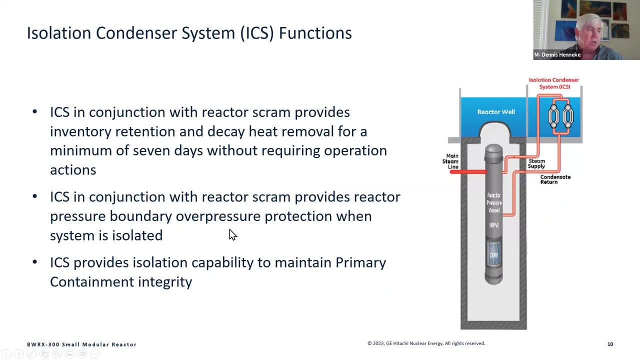 If it was to event anticipate transit without a tram, then we'll have to open up multiple isolation condensers. And again, I think I missed it on one of the previous slide that this here isolation condenser not only provides the safety function for removing heat or heat removal, it also is. 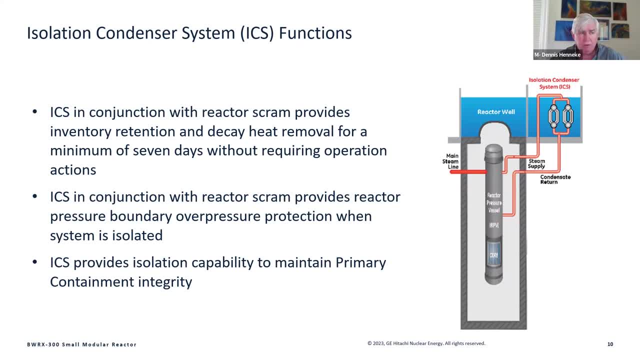 our primary pressure control. With the longer vessel, very large steam space. when a current flows isolation condenser opens, those need to control the design pressure of the vessel. There is a non-safety-related pressure relief system that's there as a defense indemnity. 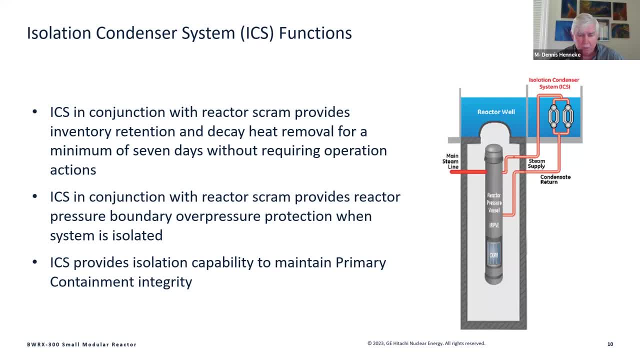 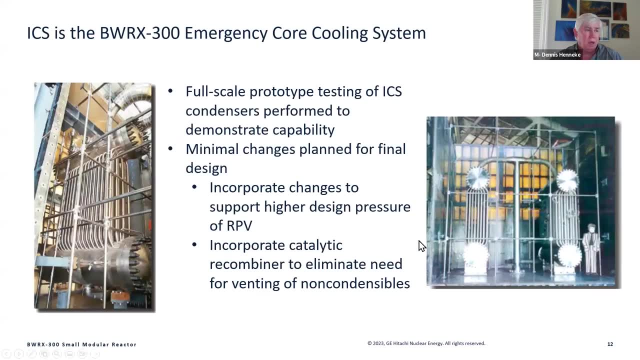 And then there's a non-safety-related pressure relief system that's there as a defense indemnity, And then there's a non-safety-related pressure relief system that's there as a defense indemnity. So the depth measure, the pressure control, is from the isolation condenser system. 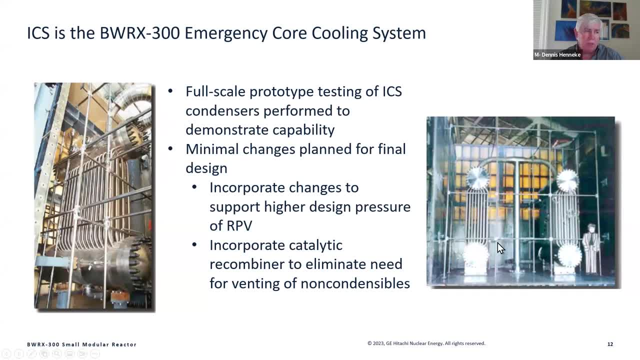 And here's just the actual isolation condenser we tested for ESP-DVR, So we have gone through prototype testing of these. There is some additional testing because we have added to the design that was not on the ESP-DVR catalytic recombiners. 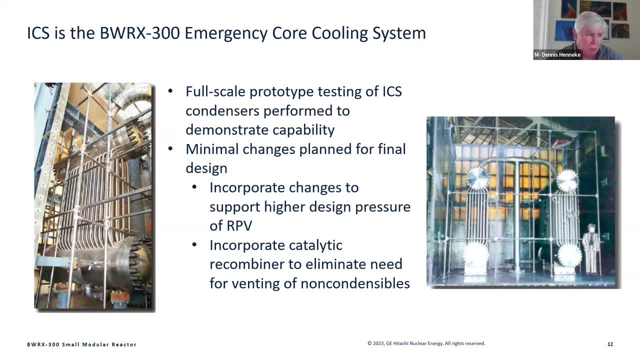 We're going to bottle up the primary and we're going to any sort of radiolytic or creation of non-condensable gases of hydrogen and oxygen in isolation condensers And so we're adding those in and we're going to have to do some of that. but that is part. 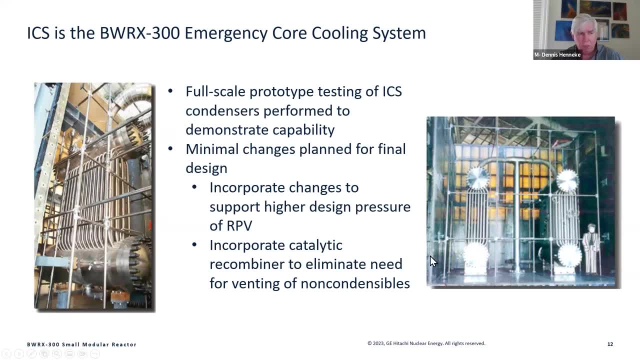 of the design. That is one of the design. the old ESP-DVR actually had a vent off the top of the isolation condensers, So we're going to have to vent off the non-condensable gas. in order to last for seven days, we need. 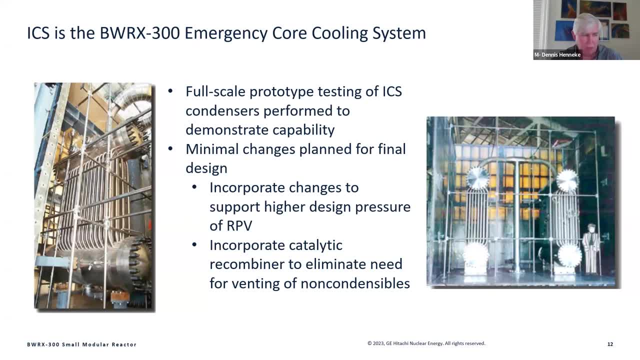 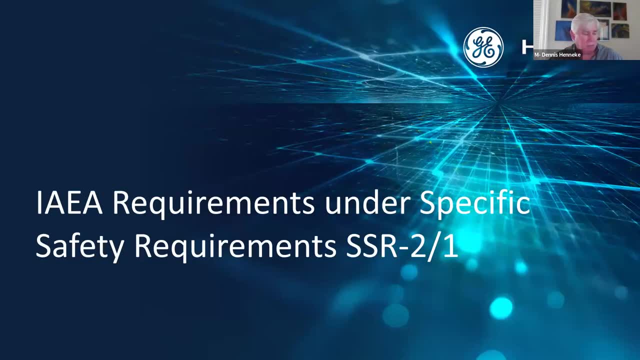 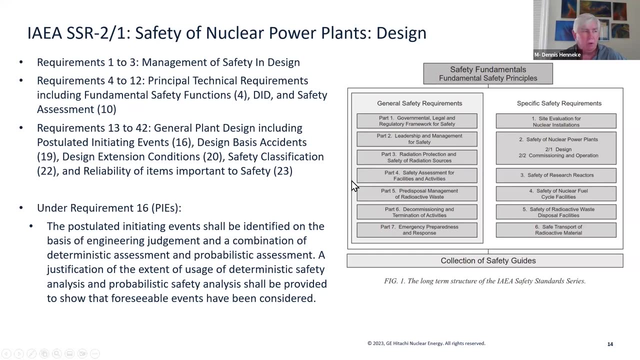 to bottle up the isolation condensers and just hold everything within the primary. Okay, let's go through the IAEA requirements, but just before I get into the safety strategy, Many of you who've heard me talk before in this area have talked about this: IAEA SSR 2.1.. 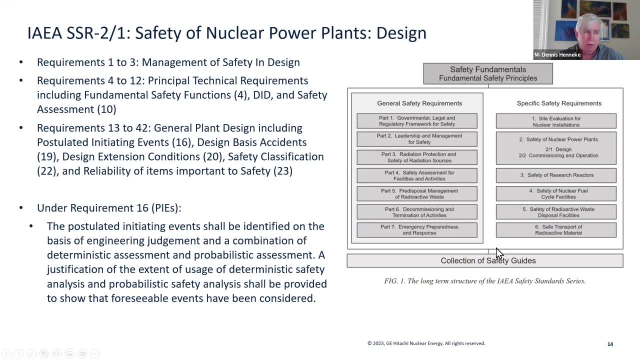 Now you see on the right side of the diagram here this is a listing or that the IAEA oftentimes presents as far as their requirements. If you're going to meet the IAEA requirements, you'll go to these documents- There are in these documents- and if you're going to meet those particular documents, 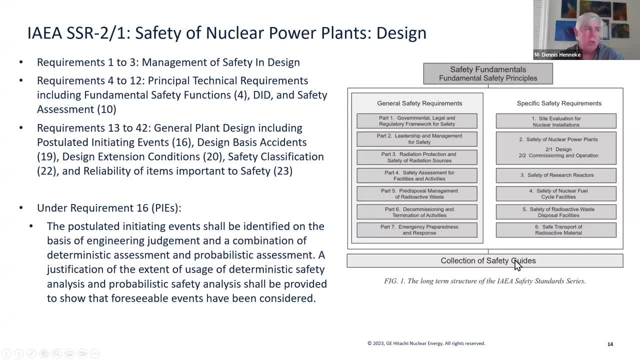 you need to meet all the shall statements that are in those documents. So you see the general safety requirements here, first of the general safety requirements documents, And then there are specific safety requirements in a series of documents, including the one that drives the safety case evaluation and design, which is SSR 2-1, safety of nuclear. 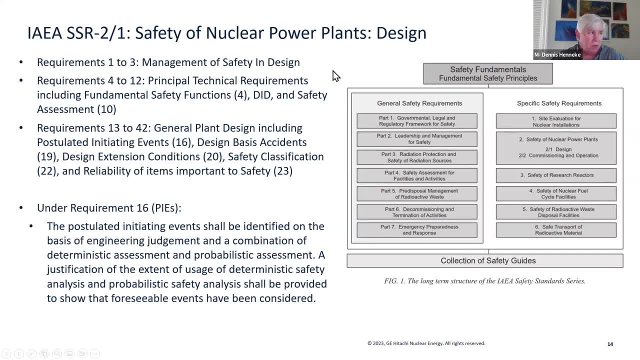 power plants in design. Now SSR 2-1 has a series of requirements and they are a series of shall, statements and with sometimes explanatory material underneath. Requirements one are the major, the high level requirements for management of safety and design. The requirements four to 12 are the principal technical requirements, which includes the 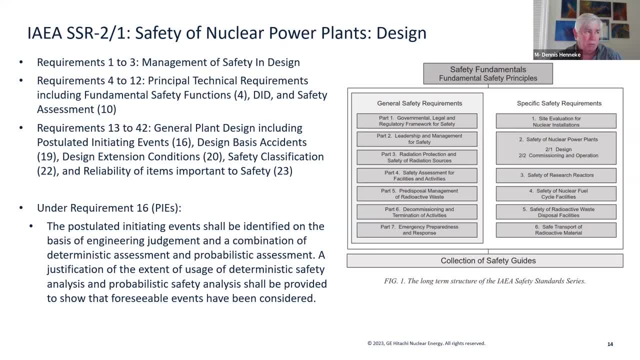 fundamental safety function development, that's requirement four. defense and depth and safety assessment, requirement 10.. And then, from there, requirements 13 through 42 provide the general plant design requirements, Including a requirement to develop a list of postulated initial events, which is requirement. 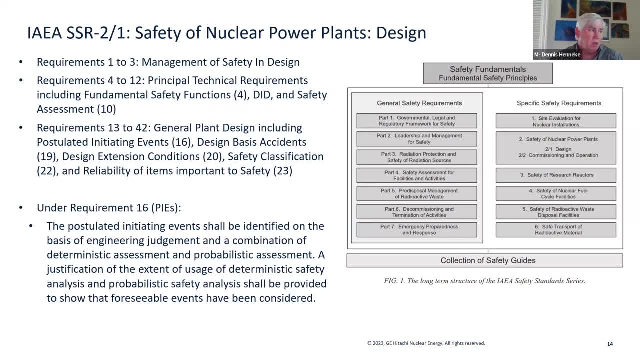 16. Analysis of design, basis of accidents, the analysis of design, extension conditions, requirement to perform safety classification and then the evaluation and verification of liability of items important to safety, And all of those requirements are part of the safety case. Of course you have to meet all the requirements if you're going to meet SSR 2-1, but all of 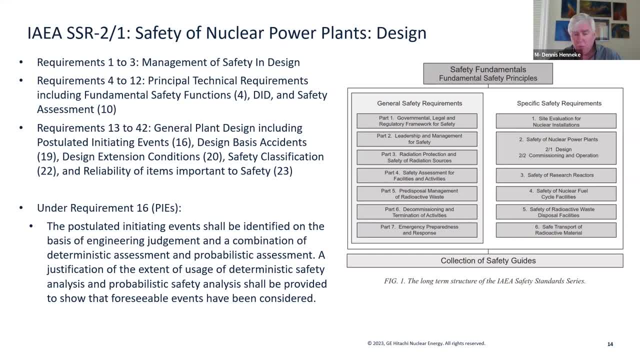 those requirements have shall statements. And I put one example here which is one of the more important aspects of a risk-informed safety strategy or deterministic safety analysis, and that's the development of postulated initial events. And in there, in requirement 16, it just says: postulated initial events shall statements. 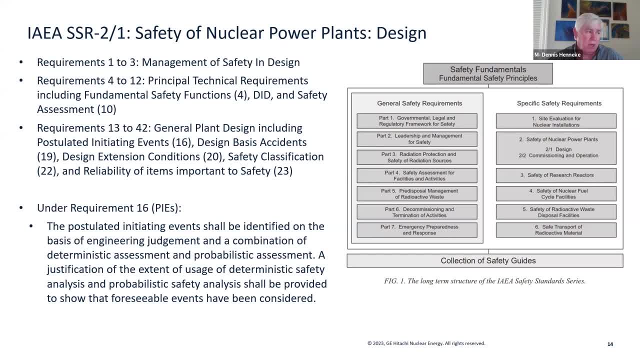 shall be identified on the basis of engineering judgment and a combination of deterministic assessment and probabilistic assessment. Justification for the extent of use of DSA and PSA shall be provided that show the foreseeable events have been considered Now, so there is a shall statement in there. 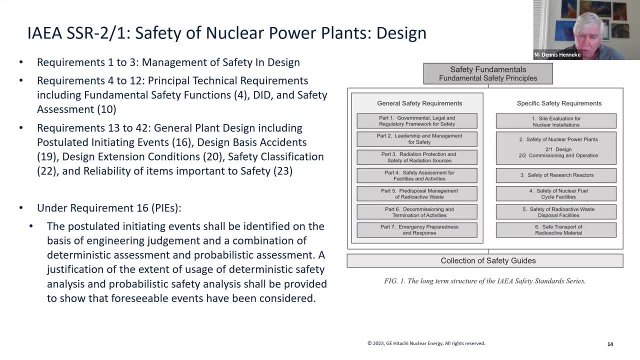 The shall statement says you have to use PSA. In fact it's SSR 2-1.. It says for plant and design- advanced plant design- you need to perform, you shall perform, a PSA. The extent of use of that in developing your postulated initial events for updating your. 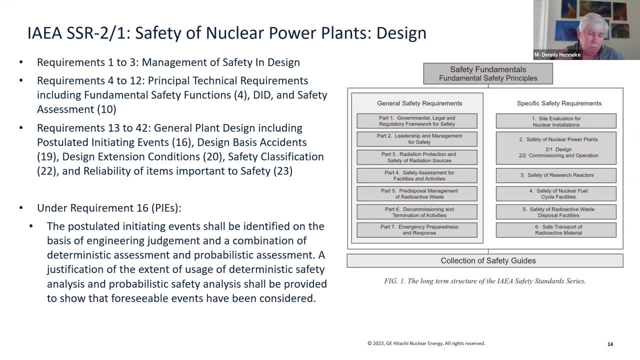 deterministic safety analysis, the performance of safety classification and so on is left to justification. In other words, you can go, you know very much risk-informed, or you can do the PSA more- what we've referred to as a confirmation basis later on- or you can be somewhere in. 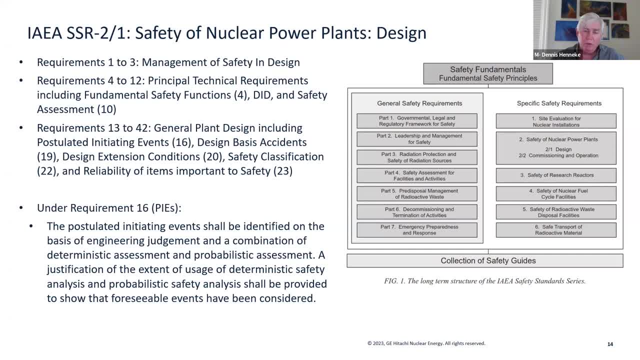 between, And I would say for GE Hitachi, we are somewhere in between. We are using the PSA aggressively but in the end the safety assessment is highly deterministic in the end And we inform the deterministic safety analysis using the PSA results. 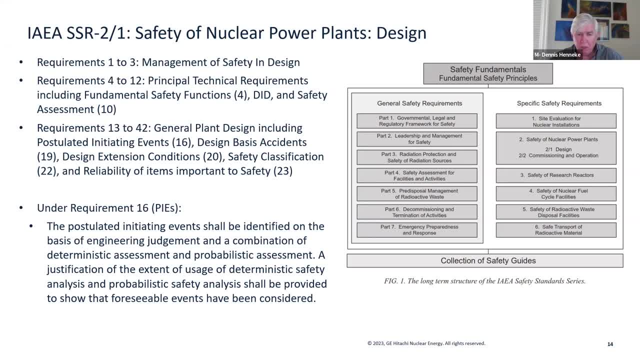 Similar to the safety classifications Based on deterministic and somewhat conservative classification. So if you'd like to understand a non-US safety case, safety basis safety analysis, feel free to open up SS 2-1.. It's not that big a document and you can read the various sections and understand what's. 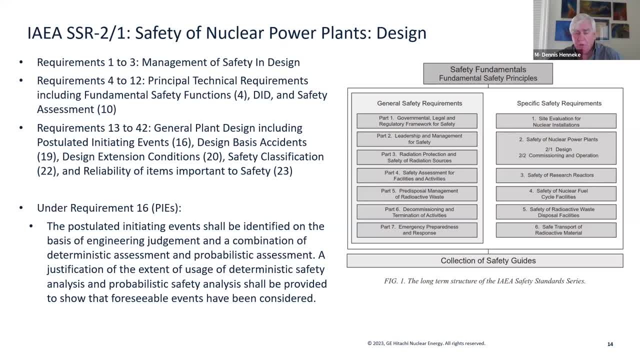 being asked. And of course the Canadians have their own- Okay- Set of requirements that bring in SS R 2-1, which are the reg docs. So they add to that the requirements, the shall statements, their own set of recommendations. 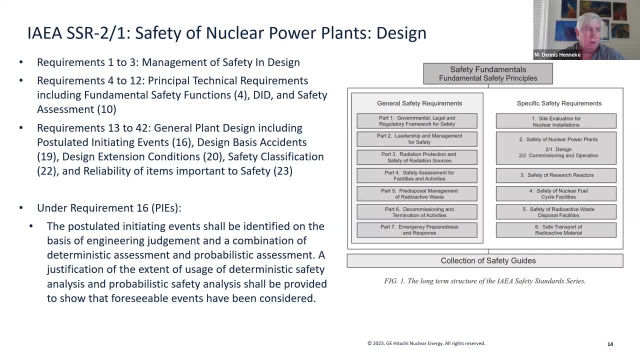 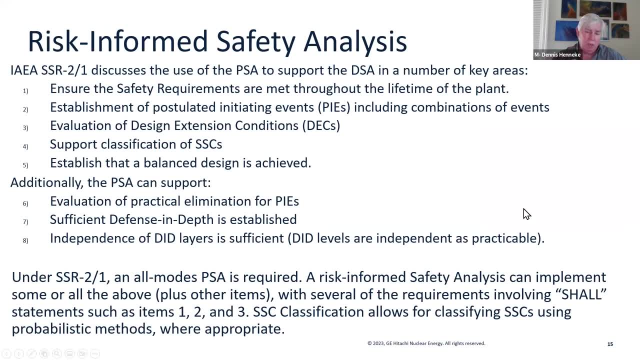 and sets of requirements, including shall statements. but that's the basic evaluation. So you can see, if you read SS R 2-1, that the risk-informed safety analysis that they require in the series of shall statements has a number of things that you can do. 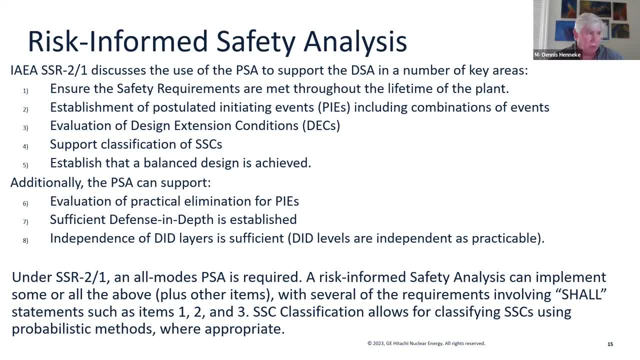 Establish the safety requirements. ensure they're met through the lifetime of the plant. establish the possibility of initiating events. evaluation of the design, extension conditions as well as the DSA safety classification. ensure the design is balanced. that that's an interesting one which we could talk about. 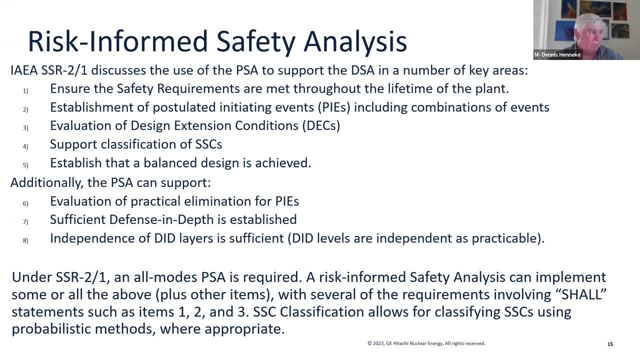 Separately, if anybody wants to talk about that one. additionally, the PSA can be used in the evaluation of practical elimination for postulated initiating events if you want to put together an argument for that. So it doesn't have to be a part of your safety case whether you have sufficient defense. 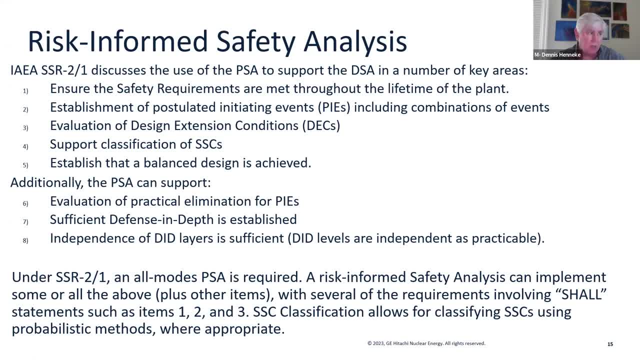 of depth and whether the layers of defense of depth are sufficiently independent. SS R 2-1 does not require layers of depth, The layers of defense, to be fully independent. they use the word independent as practicable and you can justify that and the PSA can be used for that. 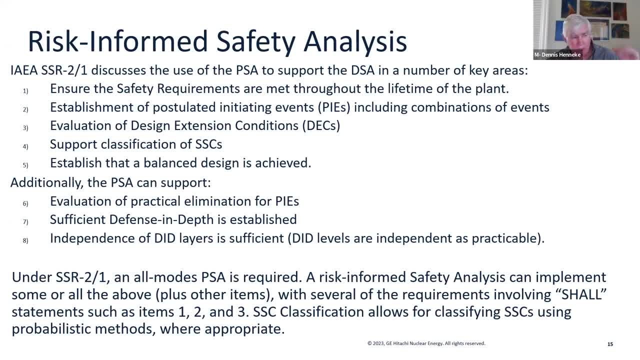 So in that the PSA, there are part of these that include the shall statements, like the possibility of initiating events, that says you shall use the PSA to support these. Definitely, items 1,, 2,, 3, and 5 are shall statements requiring the PSA. 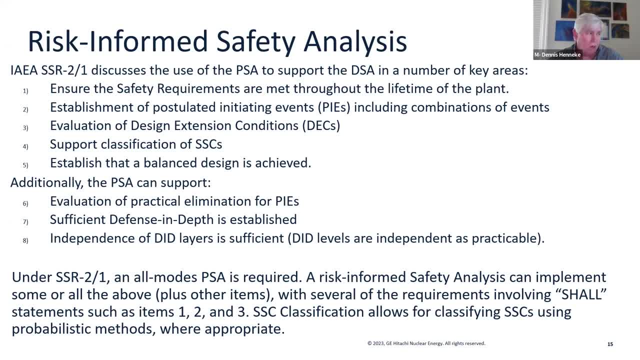 Safety classification. item 4 does not require you to use PSA. says you can use it when appropriate. So it allows you some leeway. SS R 2-1 allows you some leeway in what you will use a PSA for and what you won't. 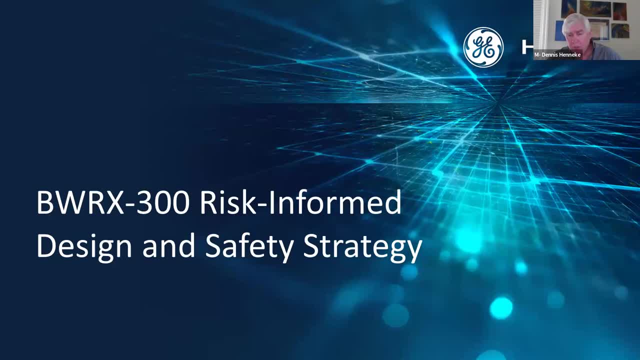 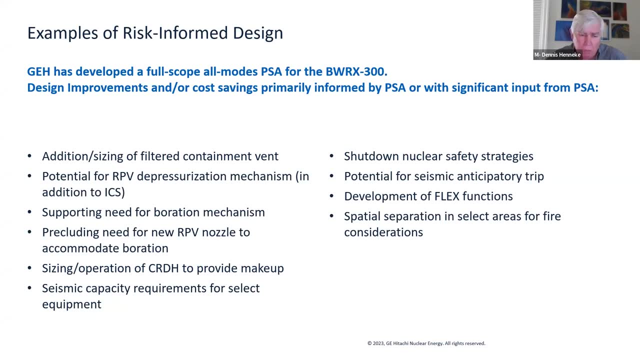 So let's get into how we implemented this at GE Itachi First. First and foremost, We have a full scope, almost all hazards, PSA. Some of it at this point in design is simplified, whereas other parts of the analysis are pretty complex. 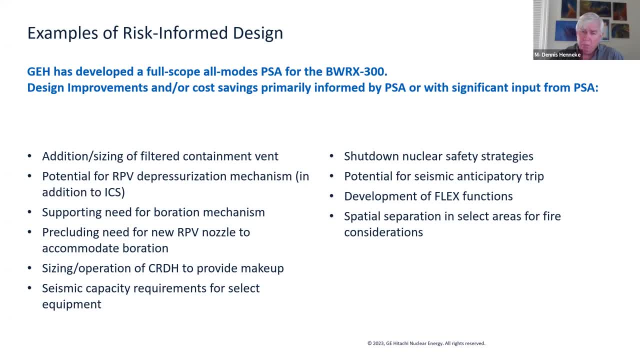 We have a seismic PSA and of course seismic- heard me say it- before- seismic winds. for advanced plants It is the higher risk of any of the hazards and it is an important aspect of our risk informed design. But since we have the PSA, we've had it for from the beginning of developing the X300,. 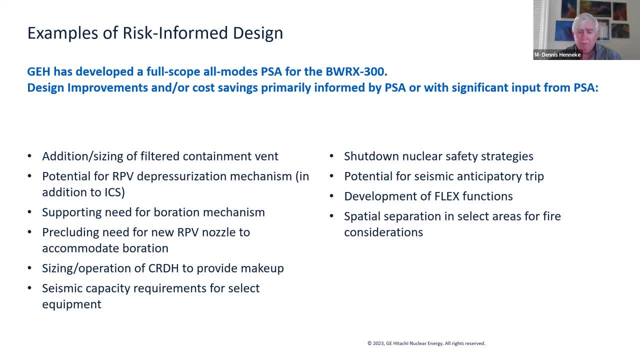 we have used it to inform the design And that's part of the first requirement is to establish design and ensure design is maintained safe throughout the lifetime of the plant. And I've just listed a few of the items here. I know Nathan DeKette's on the line. he's 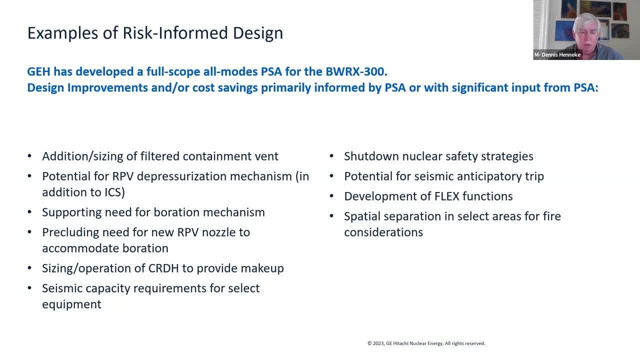 been somewhat embedded with our design team, Has worked very well with them to make sure we help, help answer questions. with regard to risk, It is not a risk-based design, it's a risk informed design. So we work with the design team to help them lower risk when it makes sense and then try. 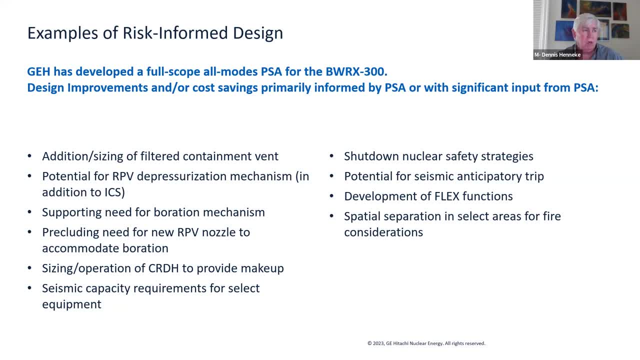 to weigh the options with regard to cost and risk when there may be a trade off involved, But the key ones, I would say: the filter containment event was important. the need for an additional non-safety related RPV depressurization mechanism was important. a boration: 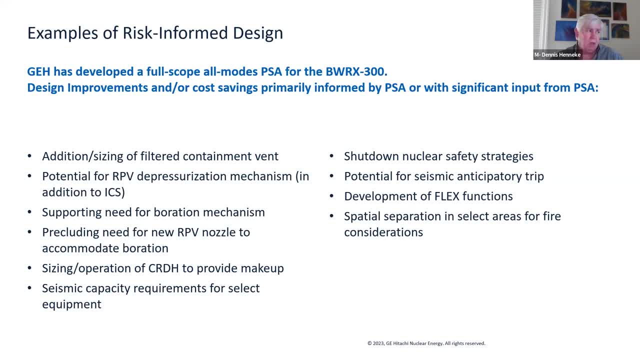 We have a non-safety. well, we're proposing a non-safety related, a boration mechanism, a boron addition, just in case there's a rod binding for all control rods. we have multiple ways to drive the rods in. But if that doesn't work, 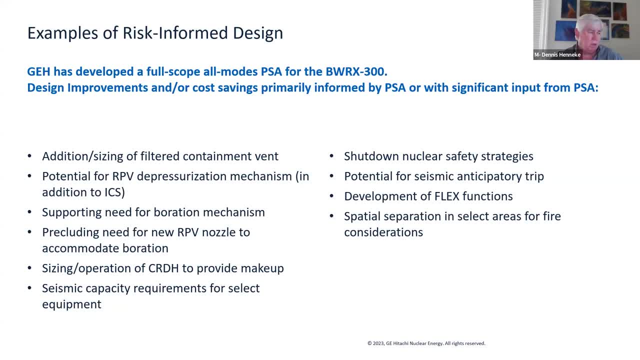 A boron addition can be used for that very low risk scenario. We have evaluated flex. it's not as important as you can imagine for an advanced plant, but we have evaluated the use of it and what functions that can provide. We have a fire PSA. we're revving it now. we've looked at some spatial separation, including 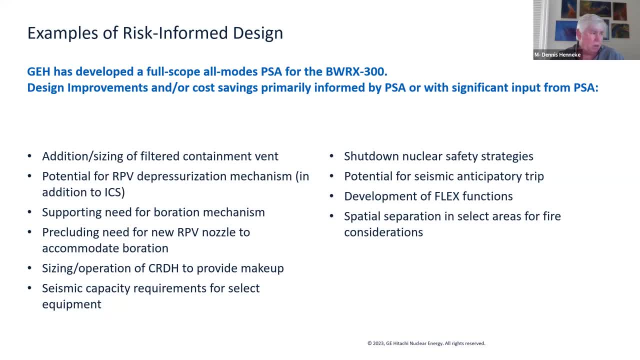 separation of non-safety related cables. And then one of the bigger items here is the bottom left: seismic capability or capacity for the. I would say there's five primary component groups with simplified reactor like the X300.. What are the capacity of those component groups? 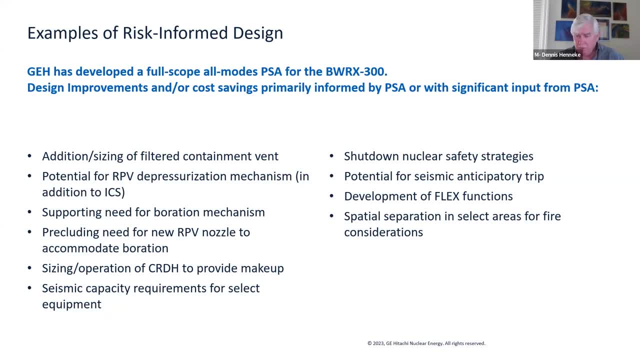 What capacity of the isolation condenser do we need, of the isolation valves for the vessel, The vessel itself, internals and containment? What capacity is needed in order to bring the risk down so that we have a balanced risk profile? so seismic isn't 99% of the risk or we're not getting close to the safety goals. 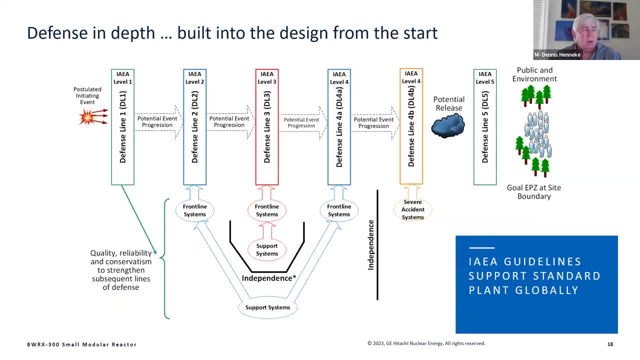 for the plant. With regard to SSR 2-1,, you'll see in there. Okay, This is a reference to another IEA document that describes the five levels of defense and depth, and this is similar to what's described in the IEA 1804: fertilizing modernization. 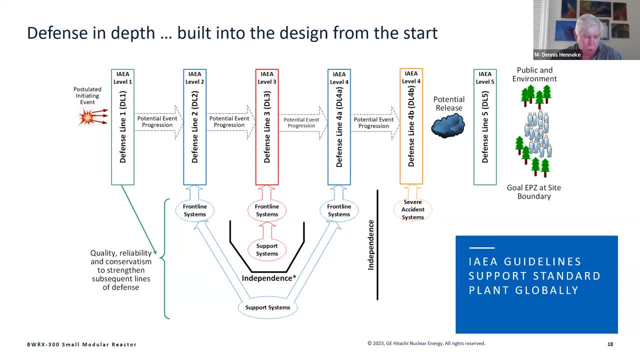 process. We have implemented a formal evaluation for defense and depth with five layers. Not all five layers are required for all postulated initiating events, but there are certain levels that are required. There are certain rules that we implement. For example, if you have anticipated an operational event, an AOL, you should have a defense line. 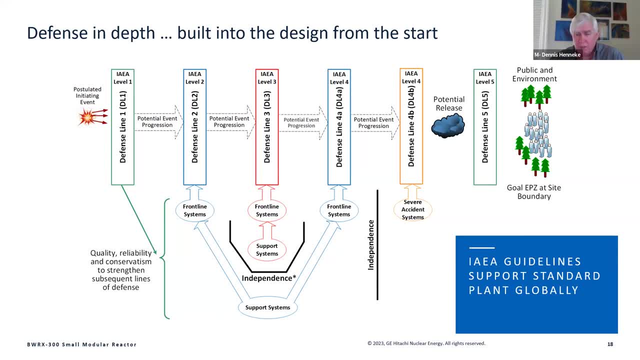 two system that prevents the operation of defense line three system, which is your safety related system. It's not a shall statement, it's a should and we try to implement it. in that regard, If you have a, If you have a lower probability or frequency event, that may be, say, in the DBA range, there. 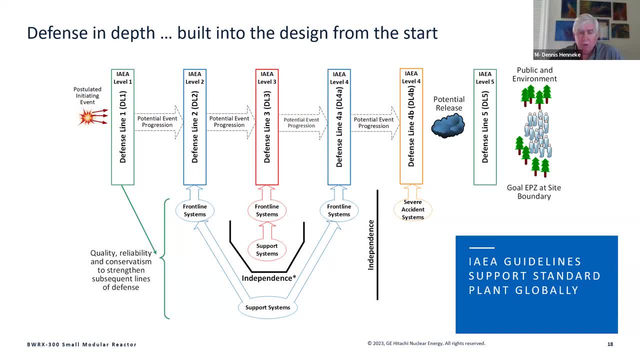 is not a requirement to have a defense level two system. We would. We'll utilize one if it's there, but you have to have a defense line three function or safety related function. Now, if you evaluate the safety analysis, what you're doing is analyzing these postulated. 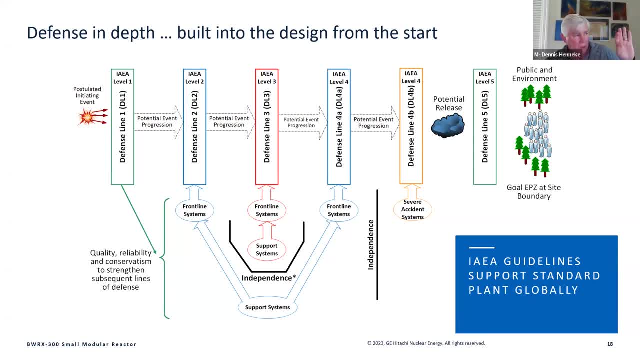 initiating events. Okay, Okay, Okay, Okay. So you have the plant response under defense line one, which are the things that try to keep your operational, Things that try to keep you from having an event by itself, but then that actuates defense. 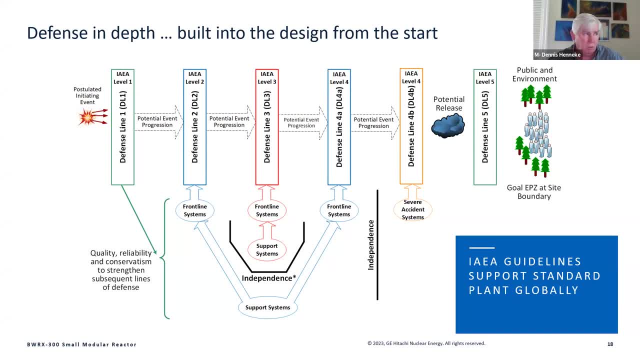 line three systems and you still have to meet your performance criteria utilizing defense line three systems, So that deterministic analysis still is a requirement, even under LMP and IEA risk-informed approach. So from there, if defense line three fails, it goes into what's called a design extension. 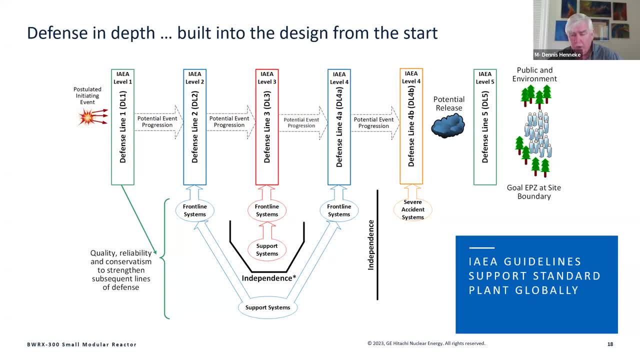 condition and then, depending on where you end up, you would have a defense line four A or four B, depending on whether you have a potential fuel damage or a severe accident event, And then, finally, defense line five is your emergency planning or flex systems, and so 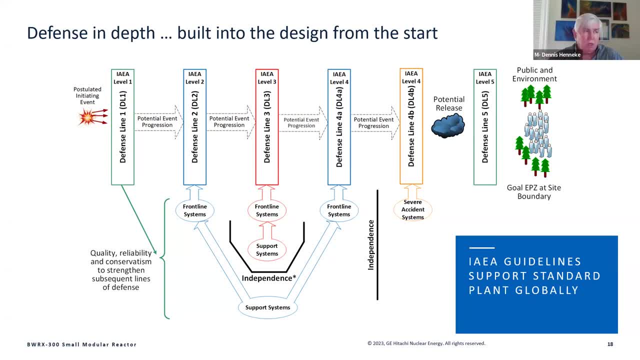 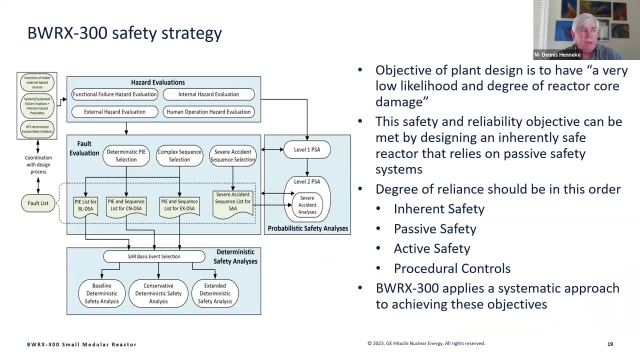 on, Okay, Okay. So that's the formal listing for each postulated initiating event and that evaluation that we utilize for all that goes into what we call a fault list or fault evaluation. This is, believe it or not, the simplified version of our fault evaluation or safety. 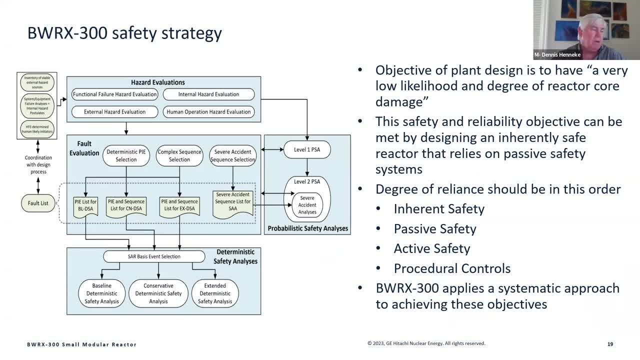 strategy that implements what I've described. Okay, Okay, And the hazard evaluations. unfortunately, under IEA terms, something would be an internal event, like a LOCA, would be a still-called hazard, or loss of feed water event, the still-called hazard. 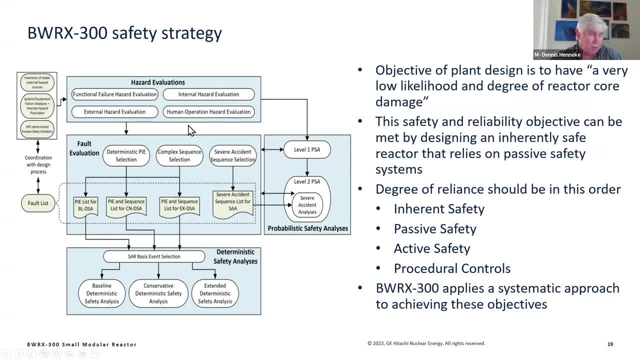 All these hazard events go through an evaluative, deterministic evaluation and a probabilistic evaluation in order to develop input to the fault list or the postulate initiating event development. Now, postulate initiating events are not just those simple events like a loss of upside power or loss of feed water event. 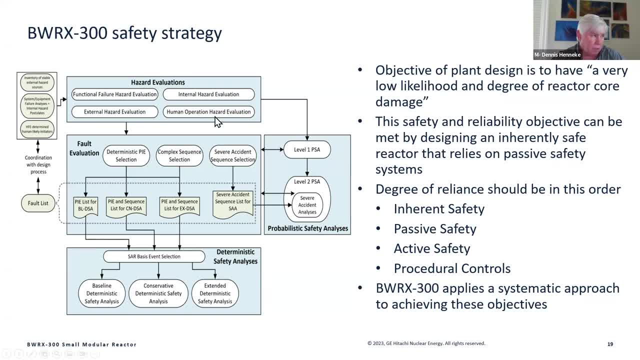 They also include other events such as shooting. They include human-induced events, all the hazard events and combinations of hazard events, and as well as complex sequence events such as loss of upside power followed by failure of all your diesels, station blackout right. 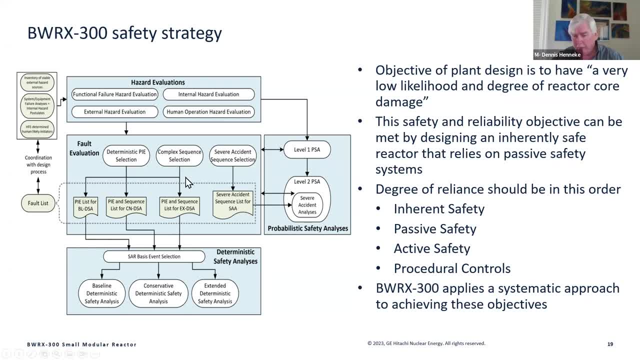 So that station blackout event or a LOCA, with failure of software, software common cause these complex sequences. we have those in the PSA, of course, but those end up being evaluated in LOCA, Added to the postulate initiating event, as complex event sequences. 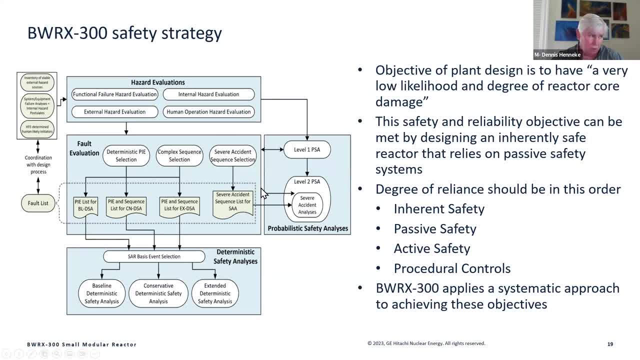 We also have severe accidents that come out of the level two PSA, that are beyond design-based, which are design-extension condition, that also go into that evaluation. So the fault list itself is a long, a very long list of potential events that can occur either in: 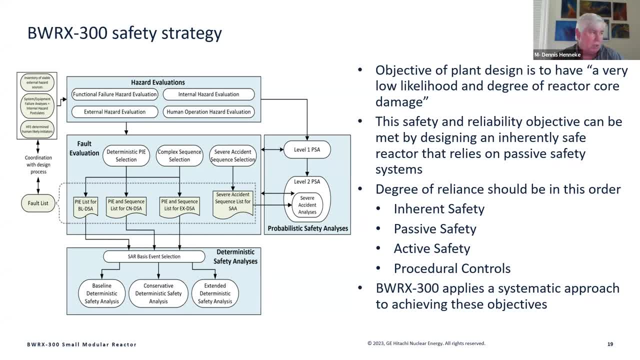 AUO space, design-based space or beyond design-based region, all the way through severe accident space that need to be analyzed within your safety case. And you can see now, although the PSA is shown off to the right, these, the deterministic and probabilistic analysis, have to work hand-in-hand and in fact they need to match. 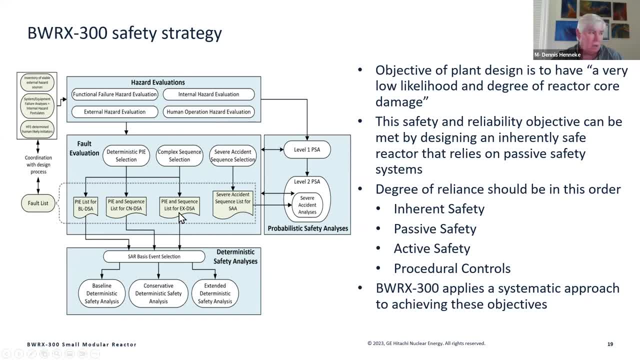 And these events, the frequency evaluation, The list itself, they need to match fully. I remember in my previous job at Duke Power I did a comparison of the PSA initiating event list versus what was in the chapter 15 of the safety analysis. 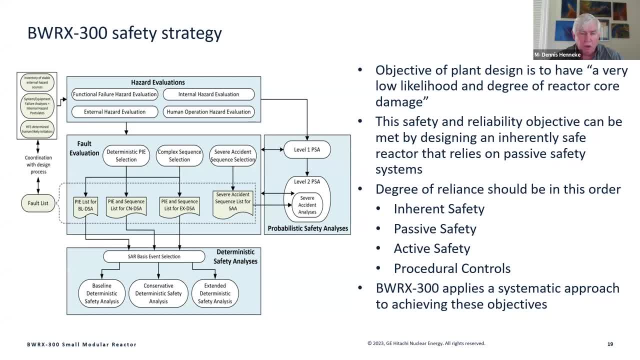 And I see some old Duke folks here and it turns out that the list was about 80% overlap. But there were some differences, But there were some differences, But there were some differences. There were things in chapter 15 of the safety analysis that were not in the PSA or the PRA and there were a number of things in the PRA that were not in the safety analysis. 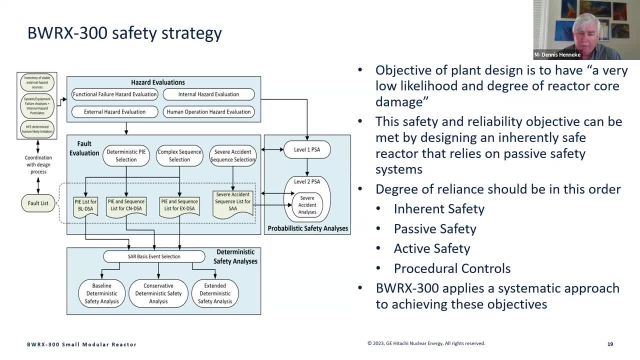 Well, we can't have that. They have to. if it's in the PSA and we show it to be especially on the design-based region or above, we have to have that on the fault list and it has to go into the safety analysis. 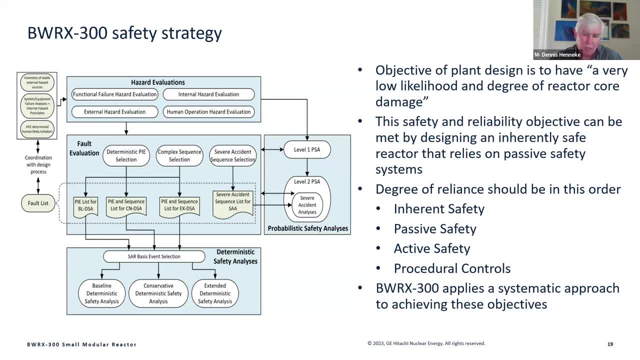 In the end, what you have is not a typical chapter. It's not a typical chapter 15 analysis. It's not a list of 20 events or 25 events anymore. This fault list is for hundreds of events. Now we can simplify that down into the PSA initiating groups, but it's still quite a large list in comparison to what we've had in the past. 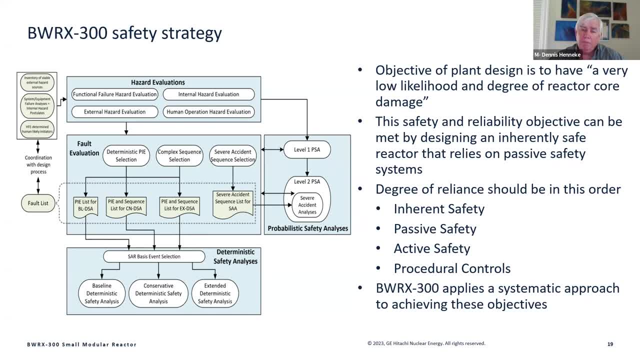 So it's quite complicated. Luckily, with a simple advanced reactor like this, the response to many of the events are very similar. So what is defense line three for one event is often defense line three for three-quarters of the events that occur. 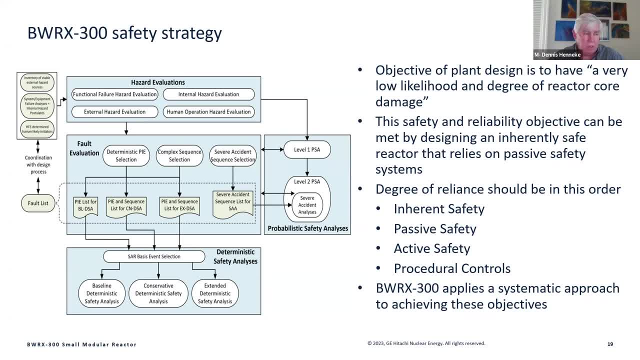 So we have a very similar response to many of the events, and we just have to make sure that those defense line three systems are capable to withstand the possibility of initiating events that we discuss, Such as high winds events or flooding events or whatever they happen to be. 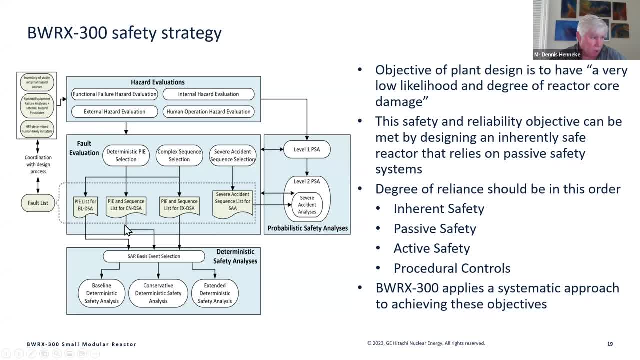 or seismic events. In the end, all of that fault list, PSA and all that that feeds into the deterministic analysis, safety analysis- which I won't go into- which includes not just a single Chapter 15 type analysis but a series of safety analysis that is performed. 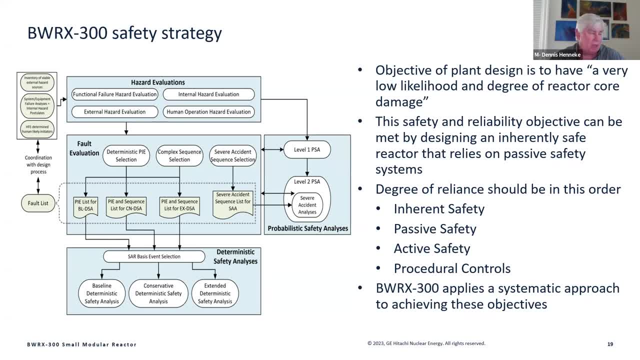 So, like I said, that's the simplified version. It's actually a little bit more complicated than that, but just remember that the PSA and the possibility of initiating event list, that's input to the DSA they have. they have to match. 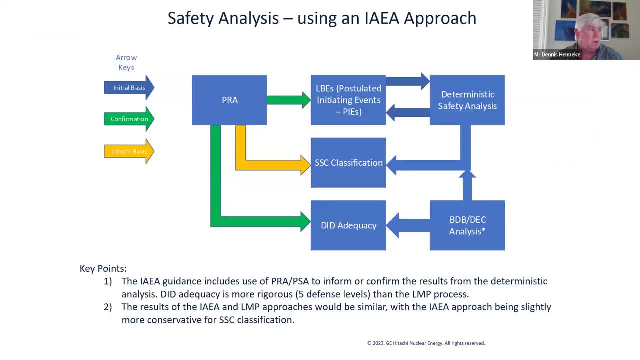 And that's one of the keys to this overall analysis. Now I created this diagram, I'll show you in the next diagram, the next page, a comparison between the IEA approach and LNP. But when you look at the licensing modernization project process, 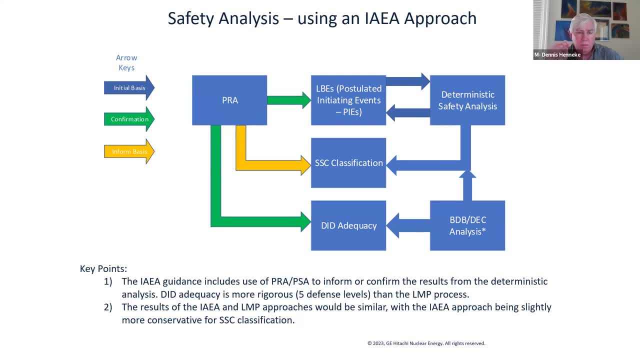 LNP process. the major three steps that we always have to go through are these: licensing based event evaluation or LISTS, which we're calling under IEA, postulating an initiating event list. Then you go through safety classification. then you do a defense in depth evaluation. 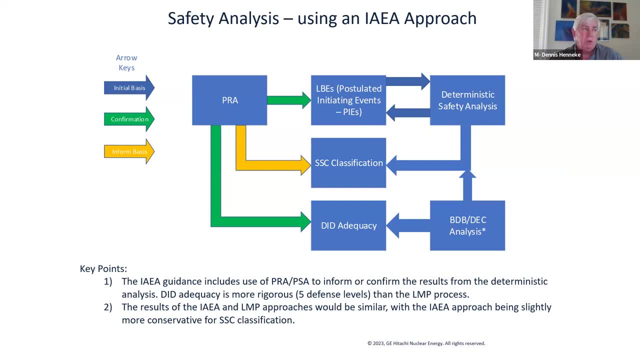 Of course you saw that there were a lot. there's a lot more to it than that. But when you look at it there, under IAEA, everything comes in and has to be justified deterministically. But on the other hand, the PSA, under IEA approach, has to confirm the PIE list. 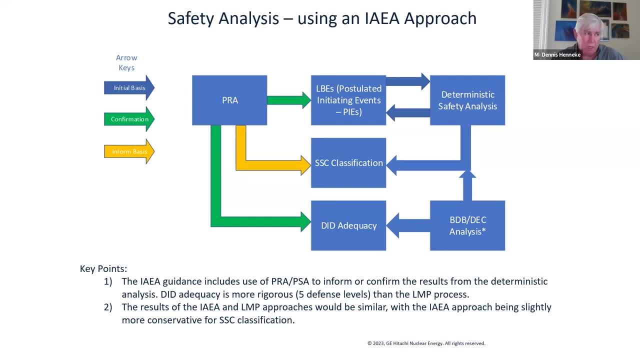 your license based event list and it has to confirm defense in depth adequacy. And you saw earlier in my earlier slide that it can be used to inform safety classification. You can be more aggressive on a risk informant standpoint and use PSA to adjust your safety classification. 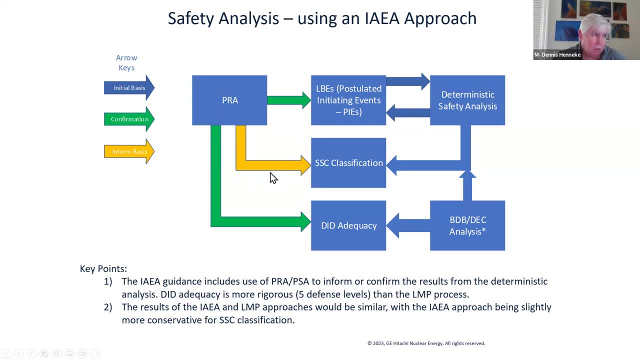 So you can turn that middle arrow on the left here from the PRA into confirmation or adjustment or whatever you want, But the base requirements are to inform the safety classification. Look for outliers. Did I miss anything? But under the IEA approach? 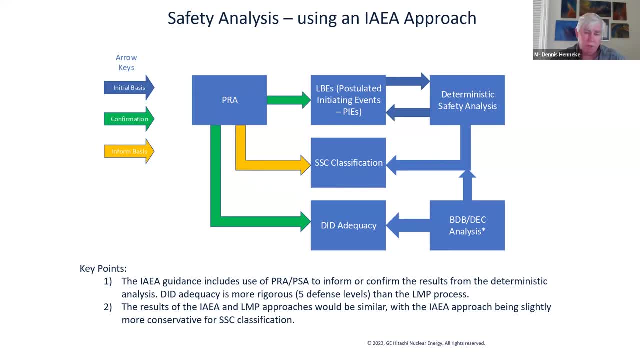 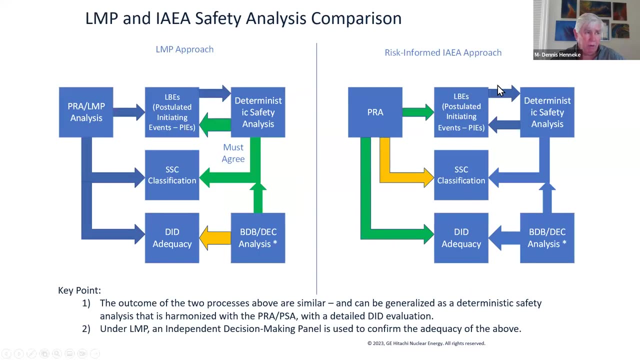 you can and you probably will be somewhat conservative on your SSE classification. So that's the three major steps we look at And obviously there are other steps, but that's kind of a one way or way to look at that If you compare that with the way we're doing. 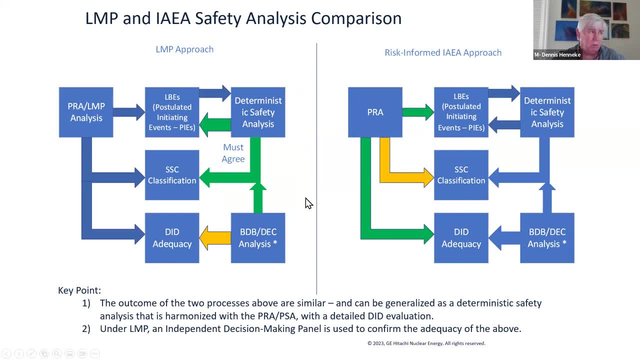 say the natrium plant and under LMP and other plants going through the lysine modernization, the PRA or PSA is used as the basis for the lysine based events, SSE classification defense in depth, with the caveat that the PSA develops all the inputs. 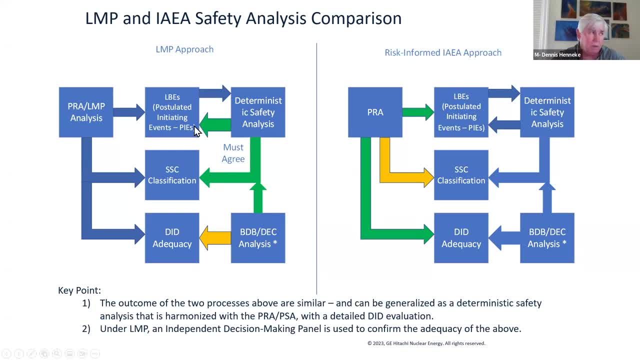 The deterministic analysis still must agree with the SSE classification so that you still have those design-based events or design-based accidents that you have to analyze and you have to show that the plant remains within the safety function requirements and the parameters are below what you need them to be in the safety analysis. 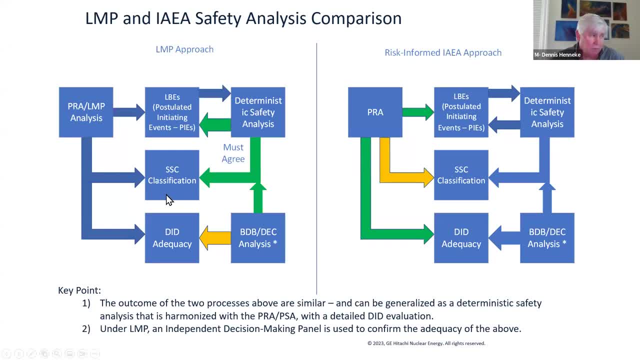 So you still need to confirm that, but still it comes from the PRA. and the other thing under LMP is you have integrated decision making panels. It's my last bullet here on the bottom- that is used to review these categorizations and agreed or confirmed that they believe those to be reasonable. 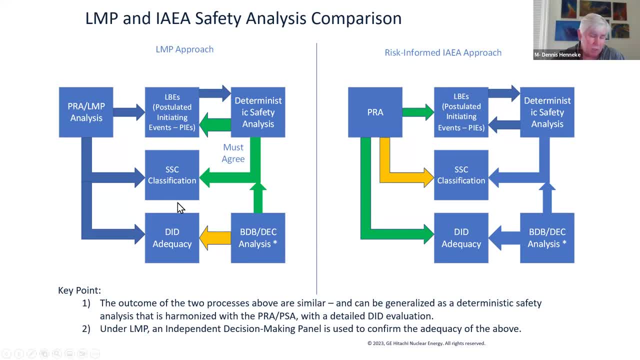 So if the PRA performs something and gives a safety classification for a component and then the integrated decision making panel reviews, views the assumption of the PRA, the scope of the PRA, and says: wait a minute, we think you're missing something here. 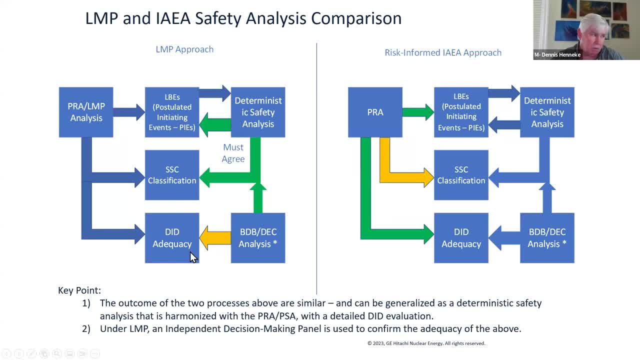 they can actually classify something higher or require additional defense or add a possible initial event for removal. So the IDPP is what makes this a risk-informed process. It's not. everything is depending fully on the PRA, But you can see the steps. 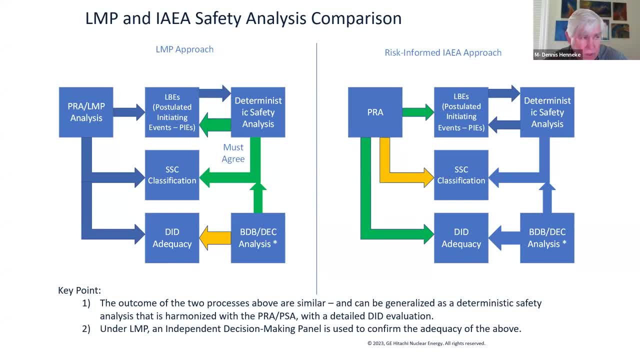 you know there's more steps than this again, but the steps are somewhat similar. but the IEA approach, the basis is fully, you know, deterministic, with a confirmation from the PRA. and the LNP approach, the basis is the. 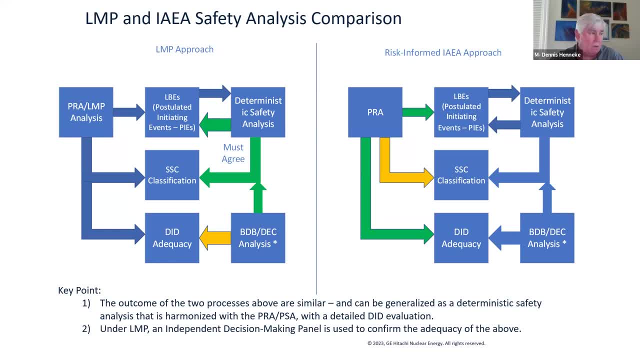 PRA with confirmation from the deterministic side. So once I started thinking about that, yeah, they look a little different, but in the end 95% of what we do under LNP is similar under the risk-informed IEA approach. 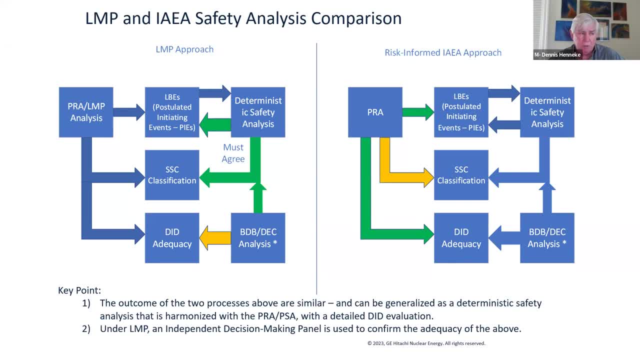 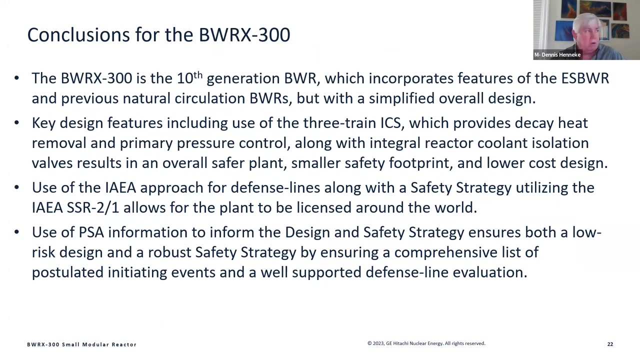 And I would say that you get very similar results with the single exception- I think I've already mentioned, is you probably get somewhat conservative SSE classification with the IEA approach over what you get under LNP. So I finished in time for questions, But you know, I think you've seen. 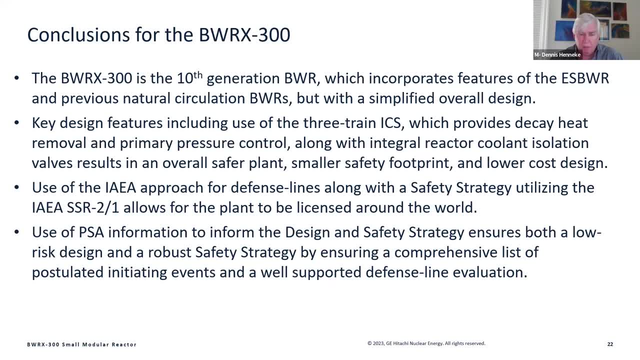 what we wanted to present here. We're excited about the X300.. We have a lot of my team members here that have done all this work and are continuing to work on this. We're all excited about the X300 and building an actual real 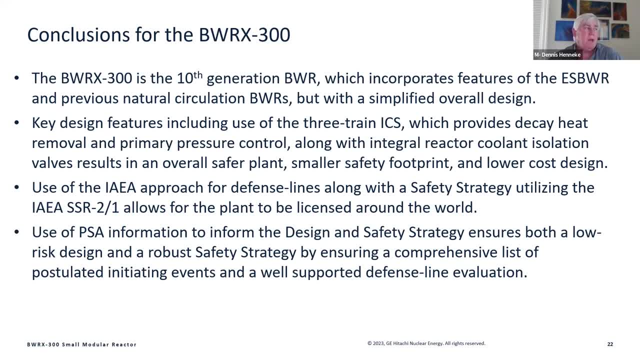 plant at the Darlington site in Canada. It's a smaller version of the ESPN NBR but it's simplified, but it's lower risk and more cost-effective. we believe And hopefully, when we build one and build the Anthropokine, that'll prove out pretty well. 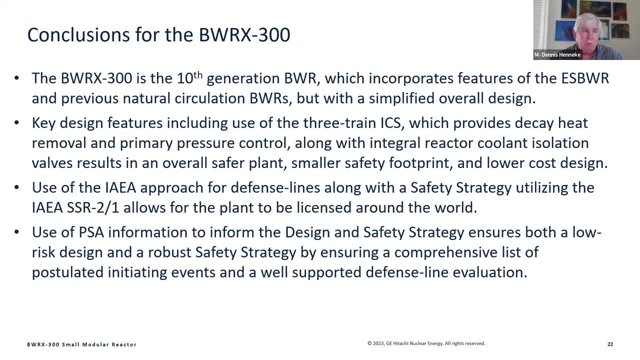 The key to design three-train isolation condenser with two return valves, normally closed that fail, open that all you have to do is open those and the isolation condenser works. That also not only provide cooling but provide pressure control. That said, since we're building out, 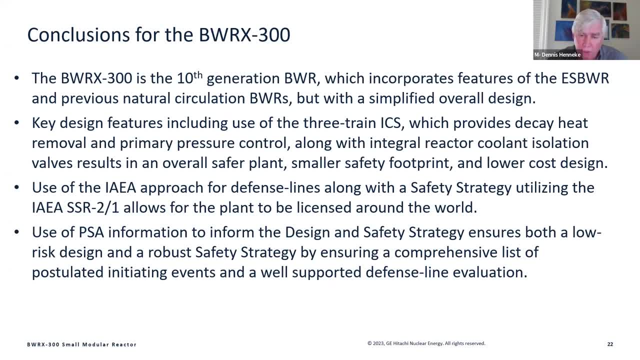 I did mention one of the reasons we're using IA approach. We're building most of our units outside the US and the IA approach is going to be something that is accepted around the world, so we're looking at plants beyond. you know the US plan. 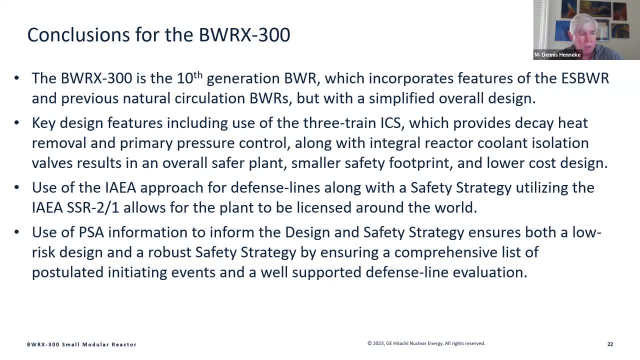 will be, hopefully, the second plant built in Tennessee at the TVA psych, but beyond that we're looking at Poland and the UK and other European countries. So So this IEA approach should allow us to take this and take the safety case to those countries and apply it throughout. 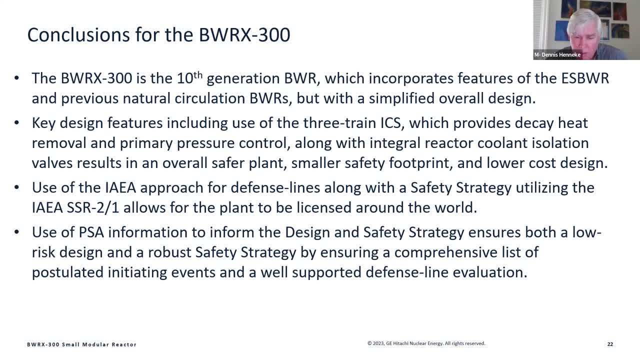 And lastly, many of you know, you know, being chair, ANS chair of JCNRM, we are, and we continue to be, PRA forward. We have all modes, all hazard PRAs for everything we do and we're pretty gung-ho on that and we're pretty excited about that. 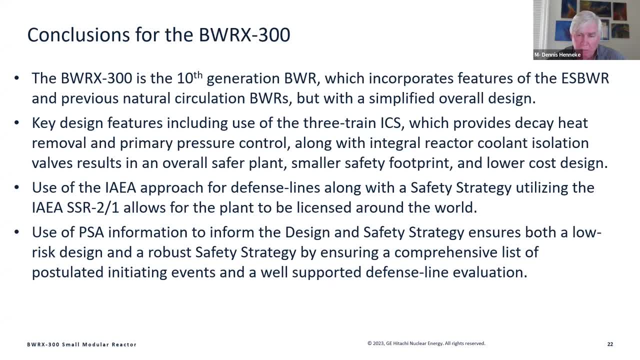 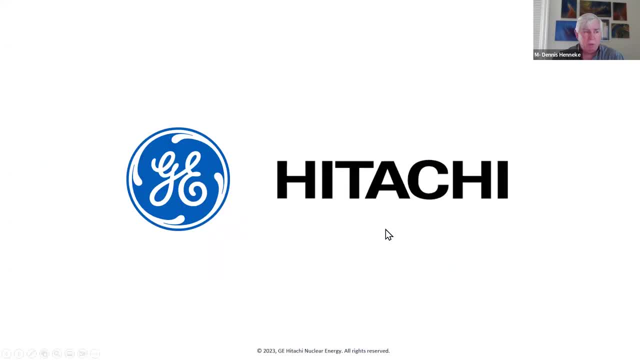 So, but that really helps us in implementing a risk-informed approach for our design. That is my presentation and I'm happy to take questions. I see Sunil, my old friend Sunil, is on. Go ahead, Sunil. Yeah, thank you. 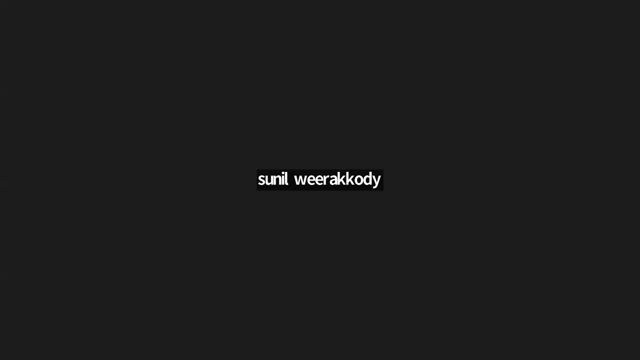 I wrote down two questions. Oh, by the way, I'm Sunil Virakudi. I'm the senior level advisor in PRA for operating reactors, But I do watch and learn about what's happening in the advanced light core reactors. So let me read for the audience the two questions I wrote. 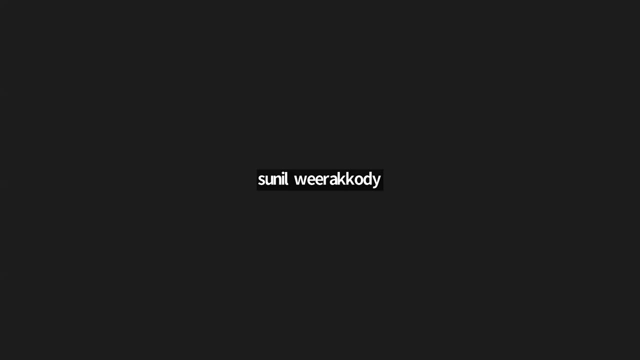 The first one is: I was asking Dennis whether he could speak to at a high level the scope and the quality requirements that you would need during the design phase to support the kind of work that you just described, Dennis. Okay, And I'm assuming it's less than what you would need further down. 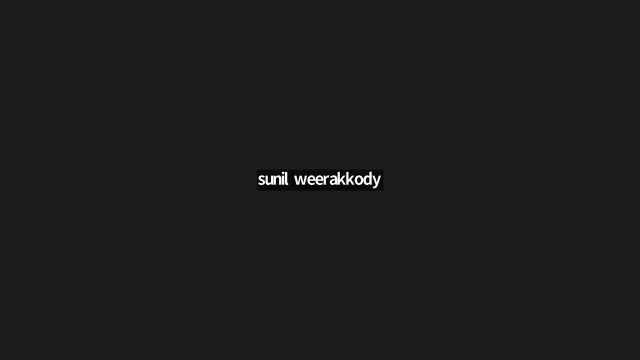 Can you talk about that and enlighten us? And I'll tell you the second question. then you can answer both. Let's hold off on the second question. Are you talking scope? Are you talking about hazards? Are you talking about level one, level two? 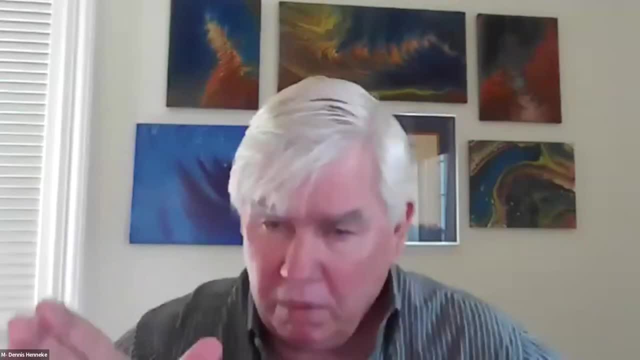 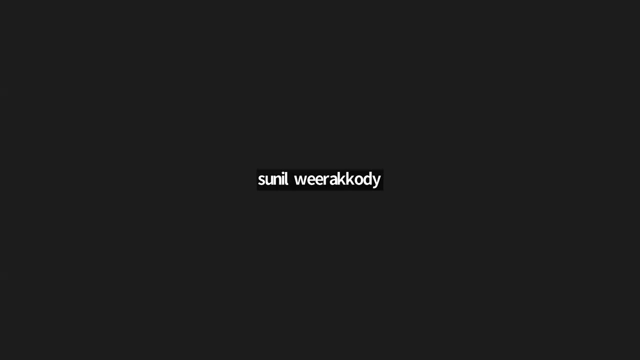 Both Yeah, Yeah. so the IEA does. in performing the PSA. it's all modes, all hazards. Okay, What you need at CP stage is up to the country. So for Canada, I think it's very similar to the US. 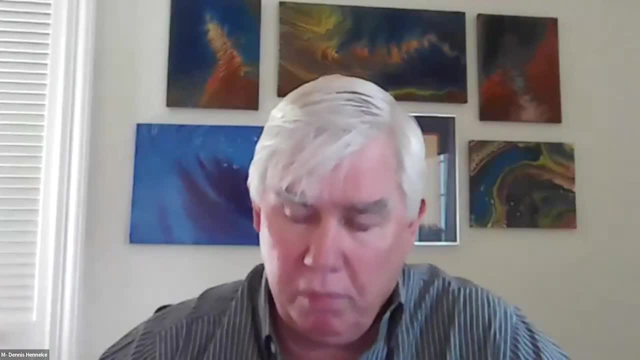 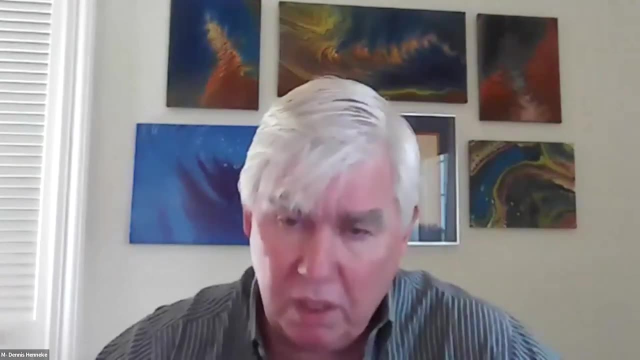 They're not requiring all modes, all hazards. We are performing it and we're doing level two And currently the IEA has no level three guidance. They've just kicked off a project starting next year for level three, but they do not require level three. 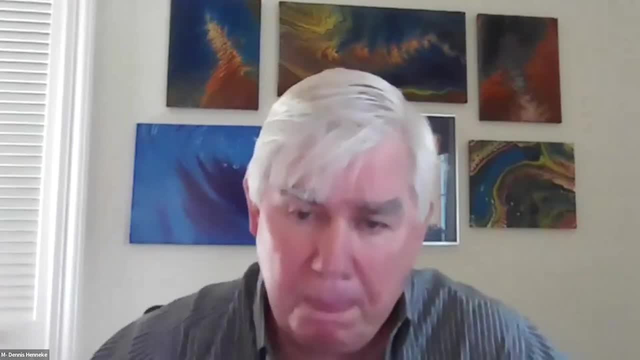 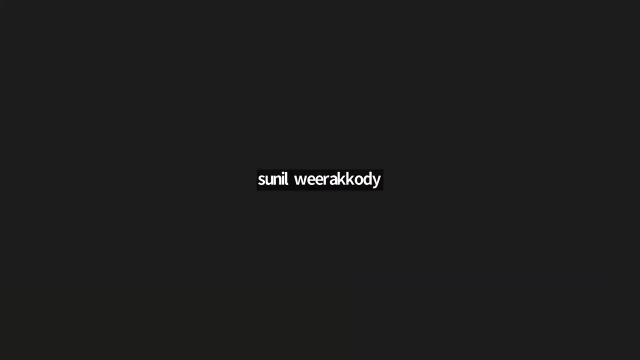 So it is level two, not lower level two, Okay, Okay, go ahead with your second question. I think you kind of answered my second question because it seems like you know, you mentioned, you know, with those two fabulous graphics, how the two frameworks compare. 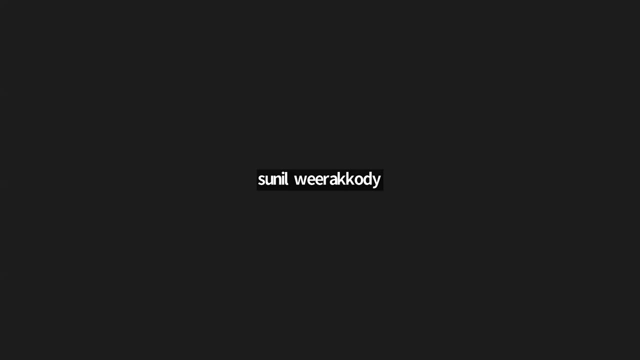 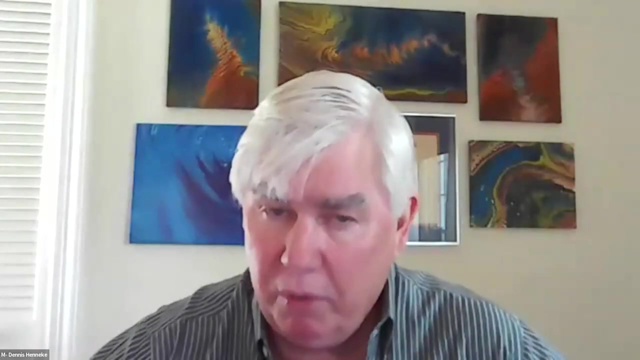 But I believe for the IEA you only require a level two, whereas for the LMP you require a level three. Have I understood it correctly? Yeah, LMP, full implementation, LMP, LMP doesn't require a full level three. 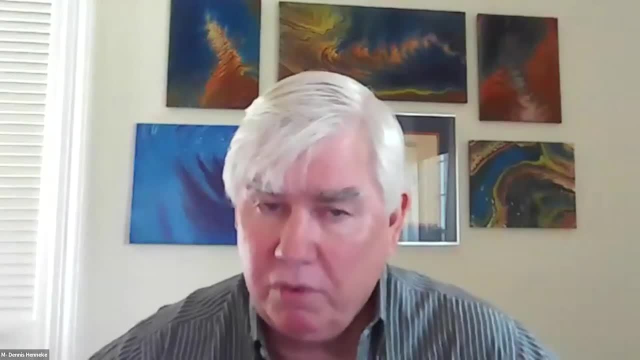 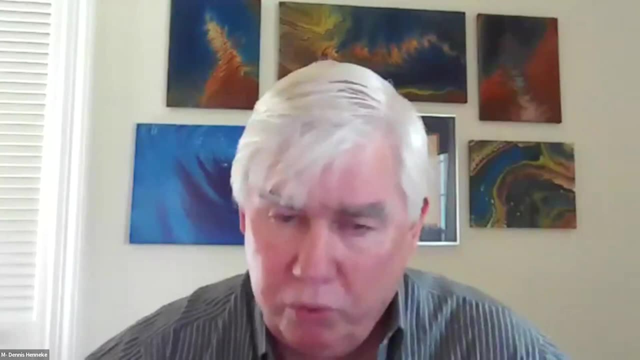 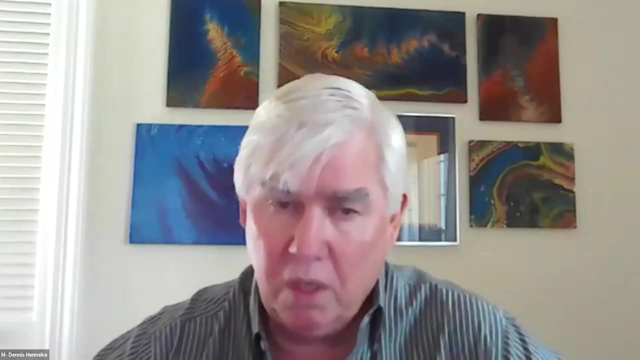 It requires dose evaluations. for off-site dose It's not. you know, you don't have to do the economic release and others. So it's a level two plus almost a full level three. So, yeah, that is a bigger difference because the metrics that you use for acceptability for LMP are definitely off-site dose. 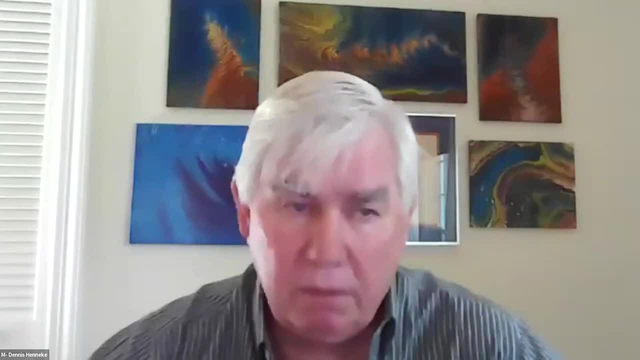 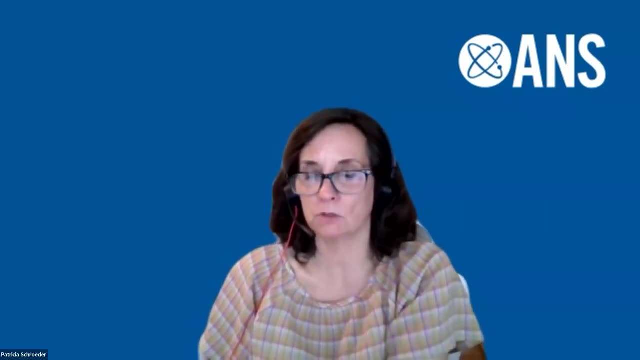 Thank you, Matt, We do. We do have some comments that kind of were in the chat before the hand-raising, so I'm not sure if you want to address those first or if the hand-raises are quick ones, For instance, like Steve Nisbet's comment has been in there for a while. 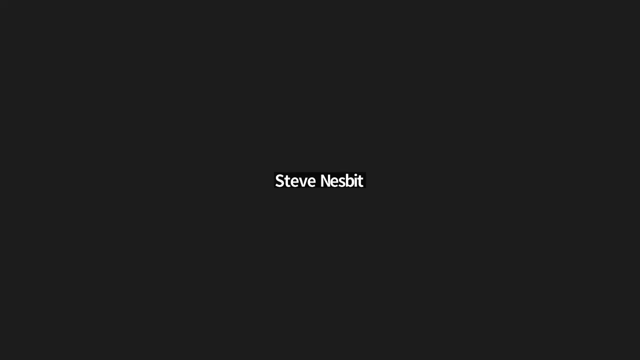 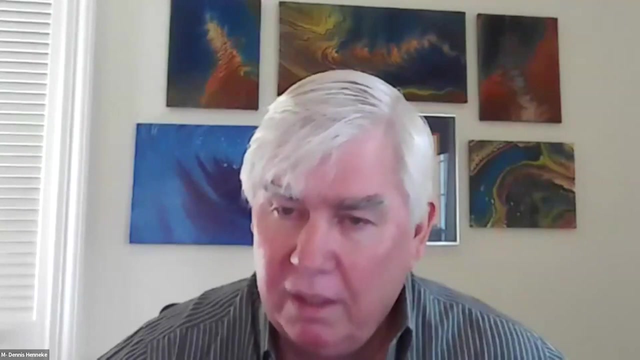 I can read that if you would like It got answered actually, Okay, Nathan answered it pretty well, so I don't think you need to go through it, Okay? So if you don't know Nathan the cat, I I've been taking credit for his work for the last two years, so he's really the brains behind all this. good looks. 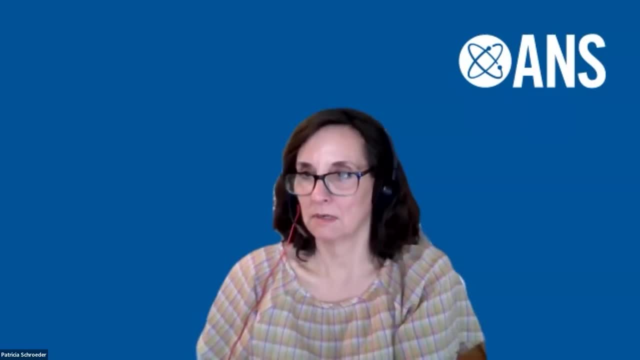 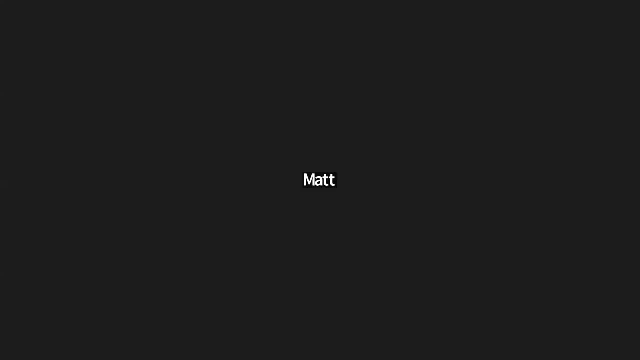 He's the brains behind it. Aw shucks. Go ahead, Matt. Thanks, Dennis, and great talk. I was curious, kind of building off the last question, What does GE view as the rate-limiting step for submittal of a construction permit at this point? 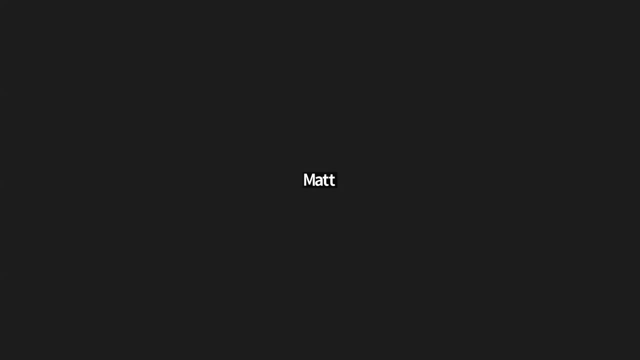 Are you Still think there's more design work to be done with the X300?? Is it still trying to round out some hazards on the PRA Deterministic safety analysis? What's the long pole in the tent as you move towards the construction permits submittal? 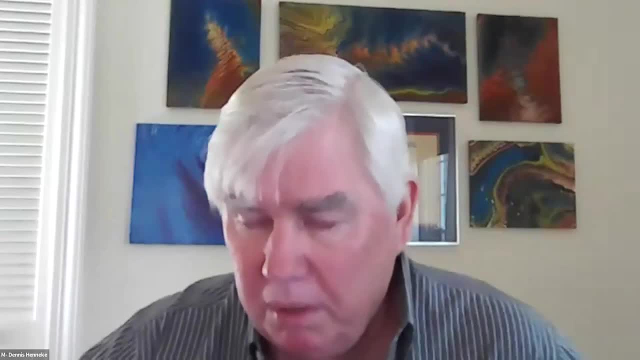 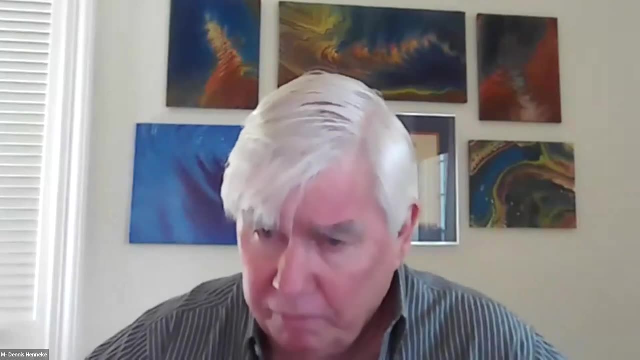 So we We submitted a construction permit for- Although it's a diet- kontrollianneahmmeH or it's a different name under it, so that would be a construction starter Canada last year. so we're already there and we continue to work, work on the. 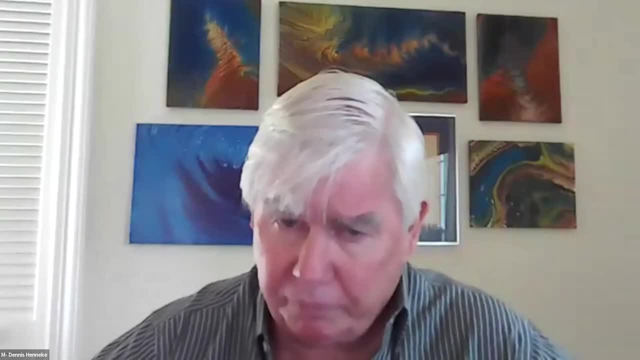 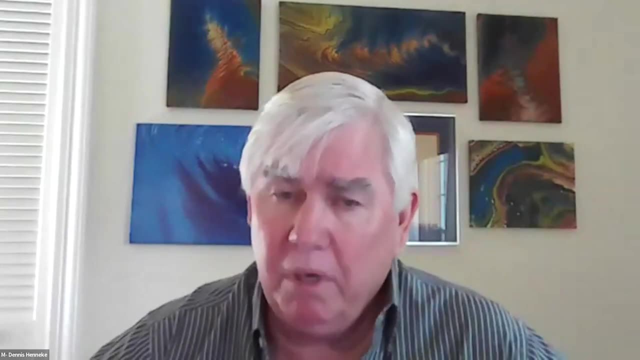 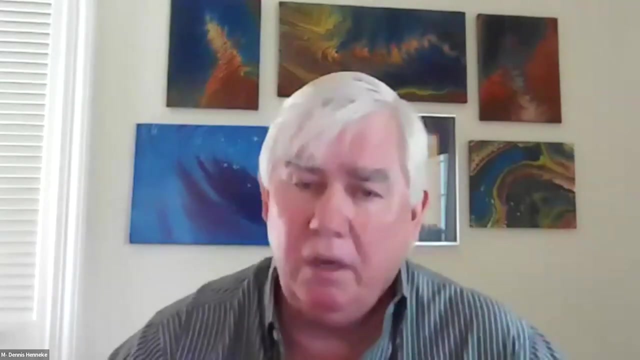 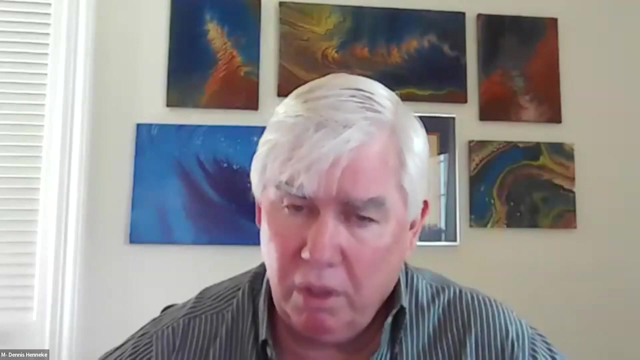 design. there there are items we have to complete, probably prior, prior to approval of the instruction permit. but for the primary are we ethical with system in the primary functions what's not designed or requirements? so, for example, as a vessel, isolation valves are pretty critical to the overall design. 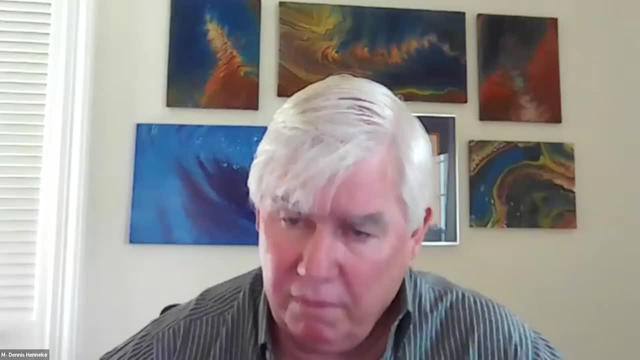 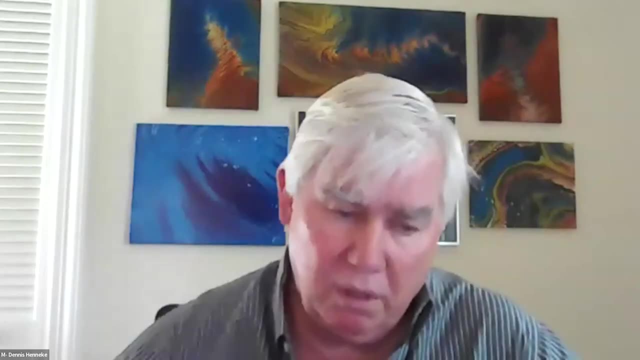 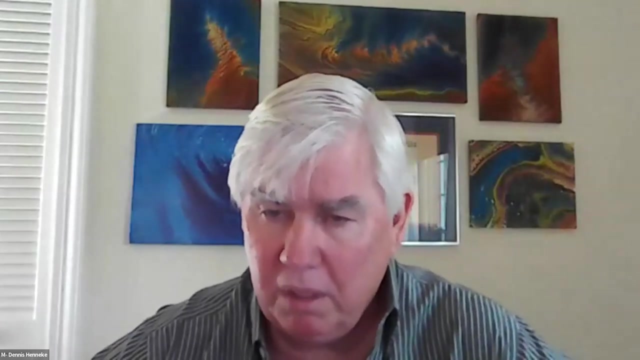 the exact design of those valves is not fully complete because we haven't gotten a vendor to fulfill the requirements of that yet to show us the exact design on those. so there's still design work continuing but we believe there's enough there in requirement space that we can submit a CP application at this stage. so 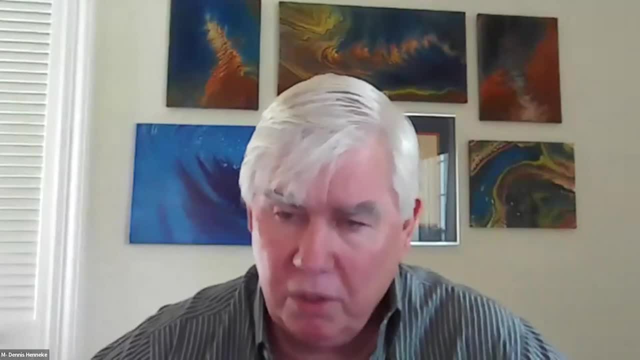 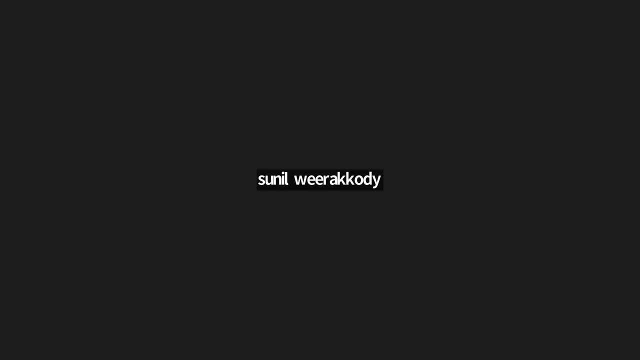 you know, people say 30 minutes is not enough, 30, 30 percent or so 40 percent, completing the design. but as far as the safety related components, I don't know what the number is. you know, Nathan, you guessed 75 percent. am I far off on that one? I was typing a. 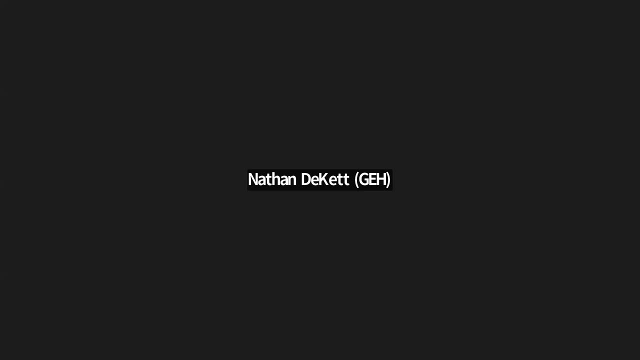 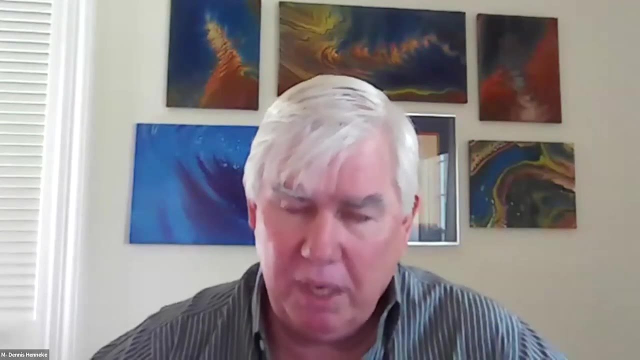 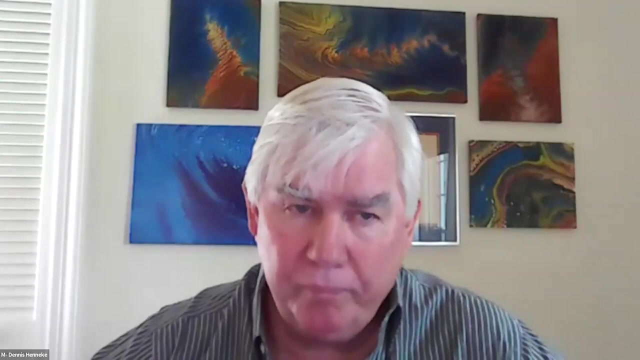 response to a chat, so I failed to hear the question. how far do you think on safety related components were completed, like for the TVA CPA, when we submit that, that, how far the safety related components will be complete in design? oh, yeah, yeah, yeah, yeah, I think that's so. it's not fully. 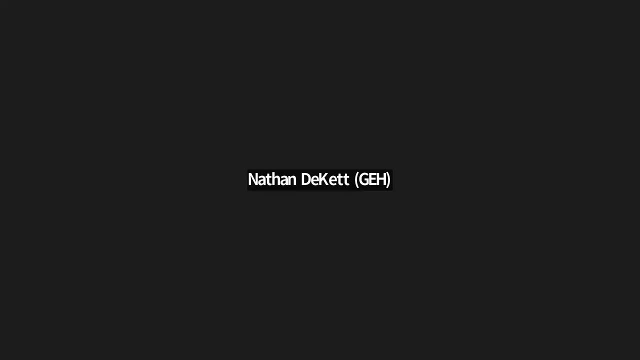 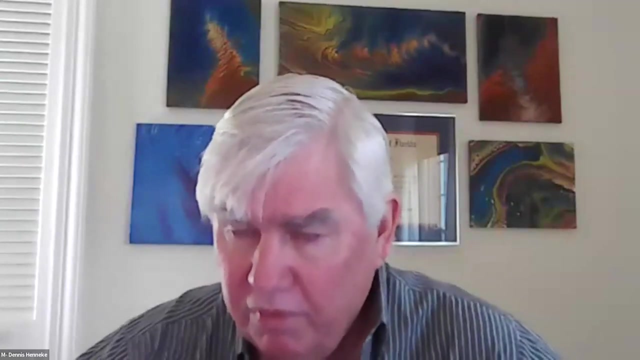 Yeah, yeah, I think that's. it's a as well, so it's not fully, not fully ilkeveted, if that makes sense, Matt. um, I'm not sure. there's a chat that you might, Billy and Pat, talk through and wait. obviously, San Diego, if you happened to taste anything. 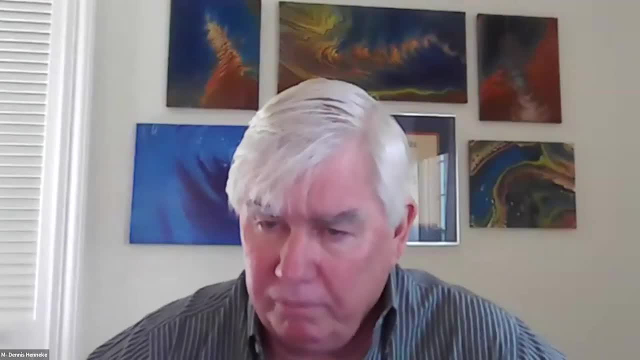 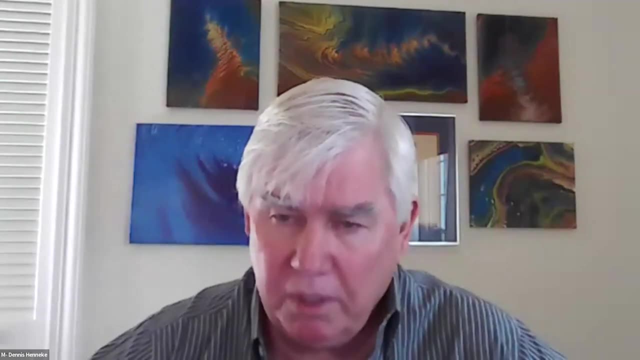 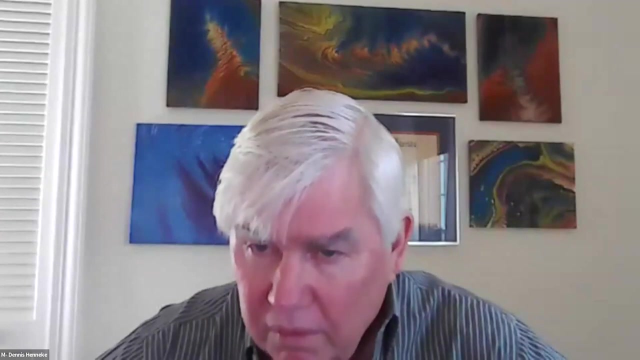 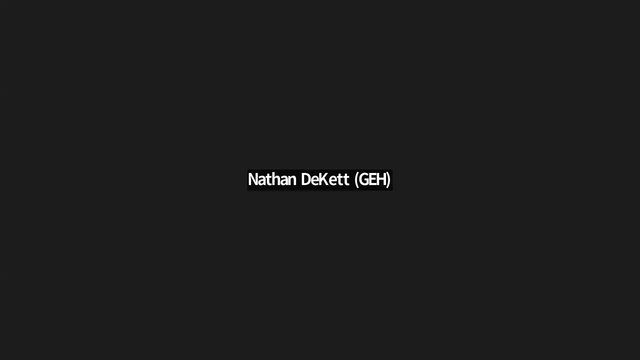 Yu biiré e. I don't know. it's not exactly accurate in the way we do it. It depends also if you're in DBA space or not. No, Nathan's already typed an answer to that, so okay. Yeah, I was trying to type in an answer to it. 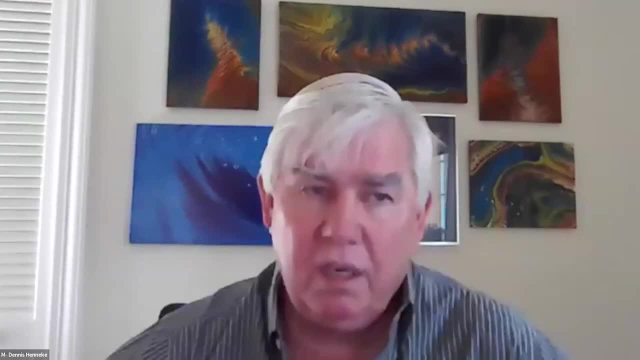 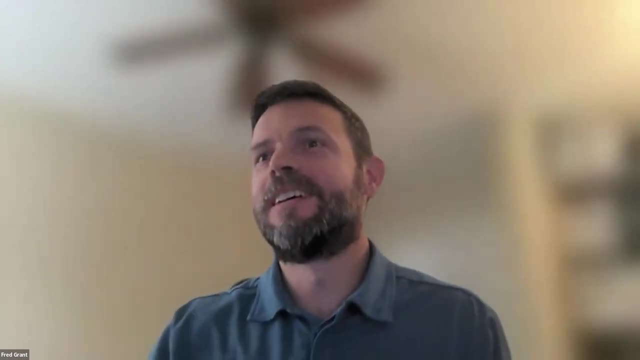 Okay, Oh, I think we're back to the hands, Fred. go ahead. Hey Dennis, Thanks for the presentation, Great presentation, Thanks. I'm interested in, you know, in using this like I guess it's- risk-informed deterministic safety analysis approach. 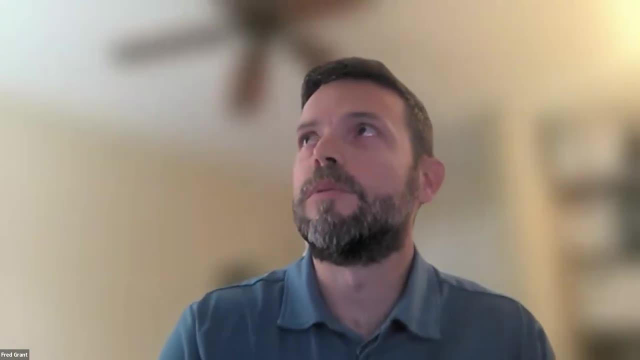 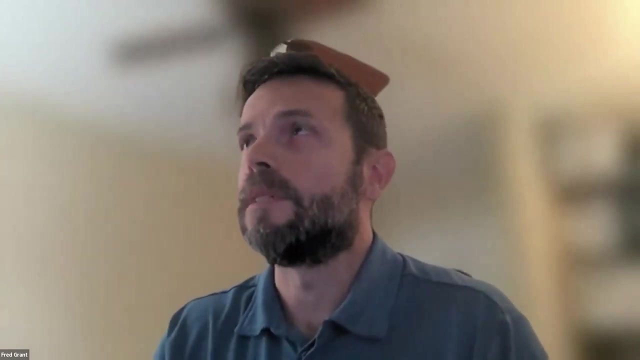 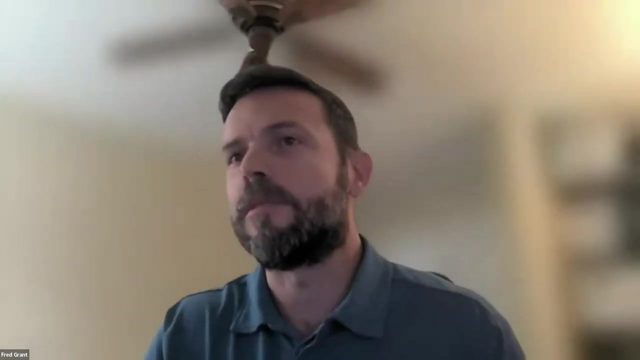 Do you have flexibility in this approach to sort of risk-informed like design, not just safety, like SSC classifications, but design criteria, like acceptance criteria, limit states, this sort of thing, Like I'm thinking seismic design here? 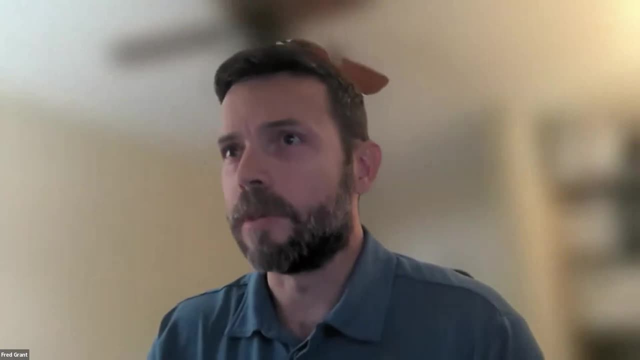 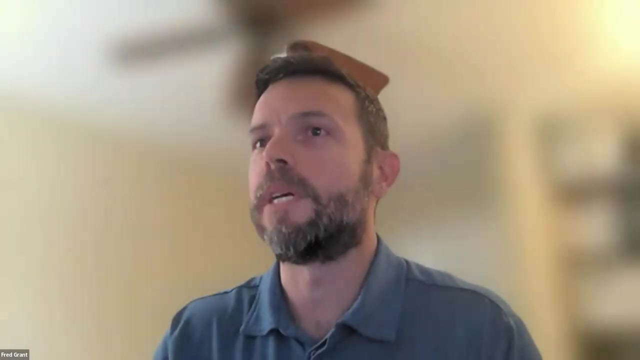 So You know you might have a reactor building that is safety-related but you know, if its credited safety function doesn't require it to remain elastic, then maybe you could relax the limit state criteria to allow some cracking and elastic behavior. 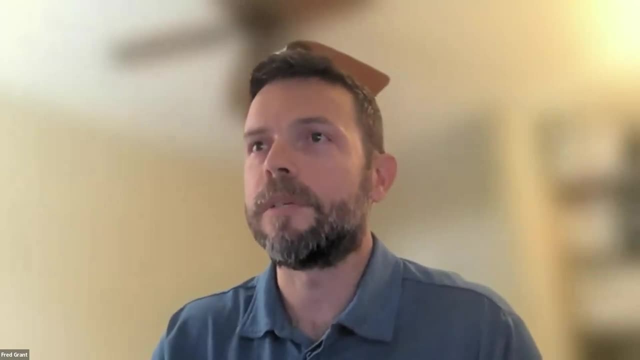 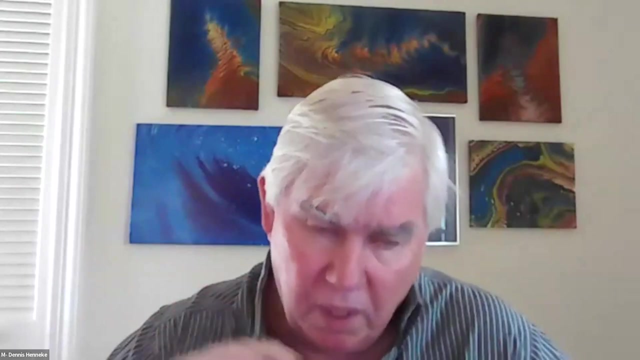 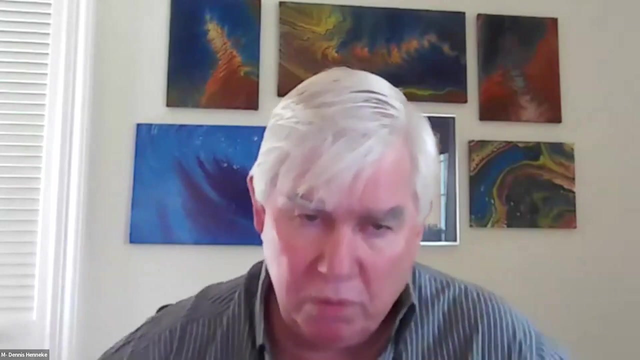 Does this method that you outlined allow that sort of flexibility? So if you saw the IEA slide, there's a series of requirements that probably not under the IEA approach you could not use risk to get away from. Those are really the higher level functions and requirements. 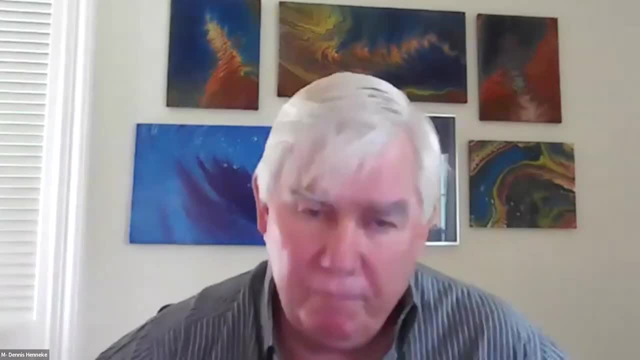 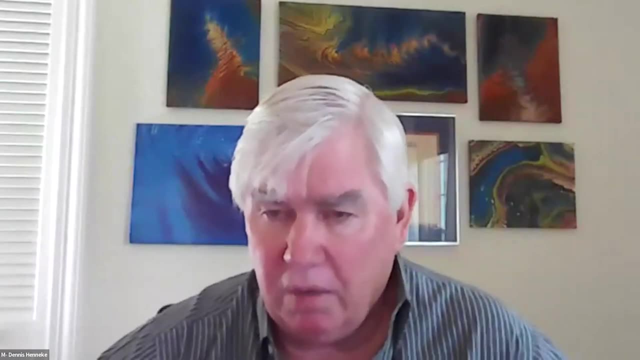 If you go down to what you're talking about, that sort of thing, that's country-specific right, So it depends on how flexible the country is. Canada falls into kind of the middle of the road. Bring me a rock, you know, provide me justification. 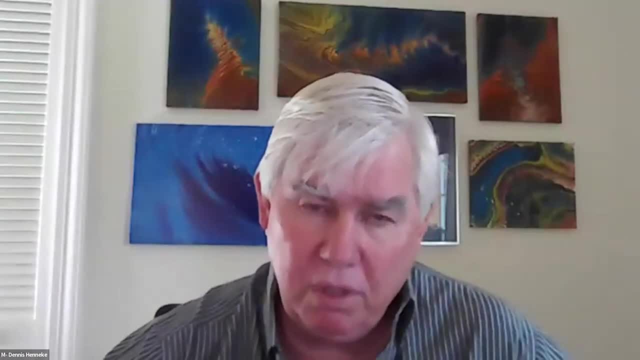 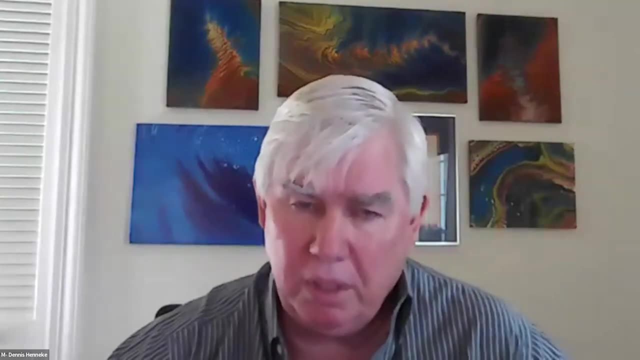 And if it makes sense we'll allow it, Except for some risk-informed changes to the basic set of requirements. So it depends on the country and the flexibility. If you were to go, take that to Finland, probably not so much right. 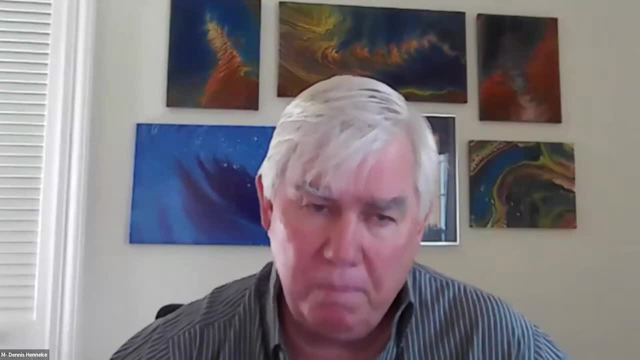 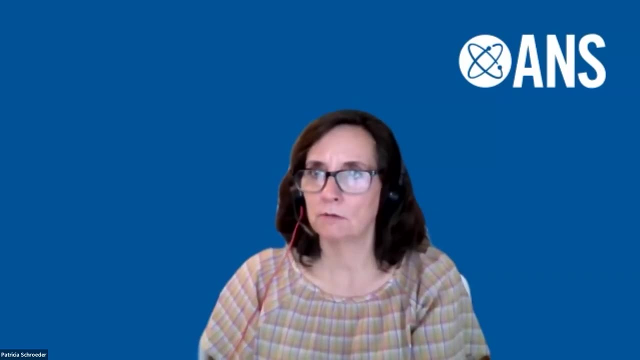 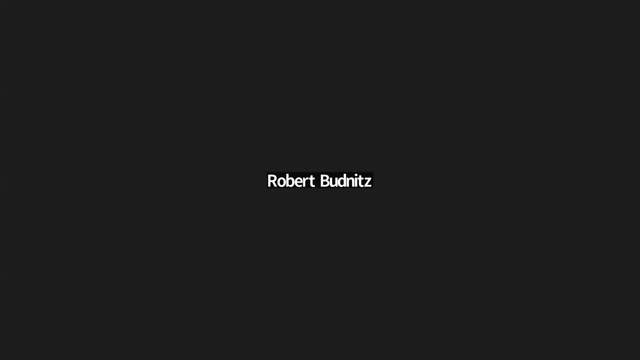 So it depends on the country. Most countries are reasonably flexible. Thanks, Appreciate. it Looks like Bob Bunditz put his hand down, Not sure if that was intentional. Yeah, Fred Grant asked my question. No, Well, we have a couple more minutes. 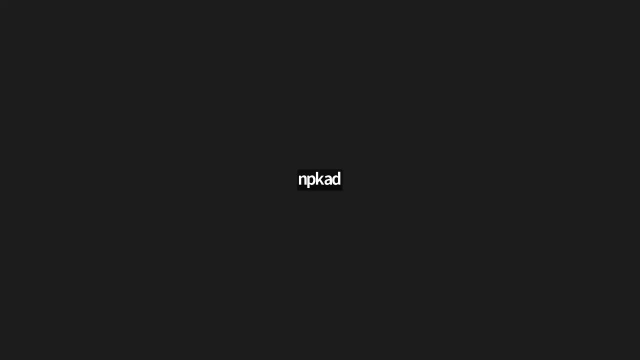 Any other questions? Well, Pat, can you hear me Very well, It's fine, Dennis. thanks for the presentation And thanks for everybody to carrying forward this program while I'm away in India. But I just wanted to point out, Dennis. 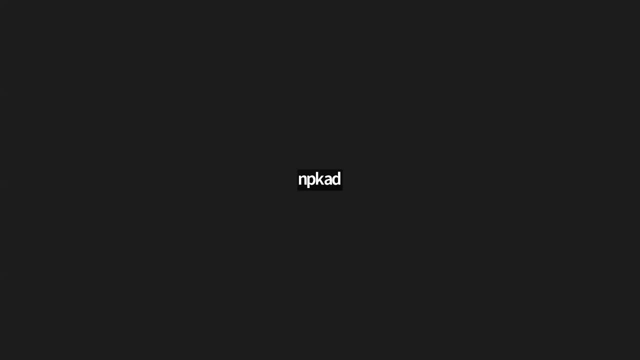 that the context, the connection between the risk-informed and the performance-based approaches, that where all this design requirements in the BWRG, BWR design focuses on reliability in your safety case, you can construct the same safety case using margins- margins to acceptable levels of performance. 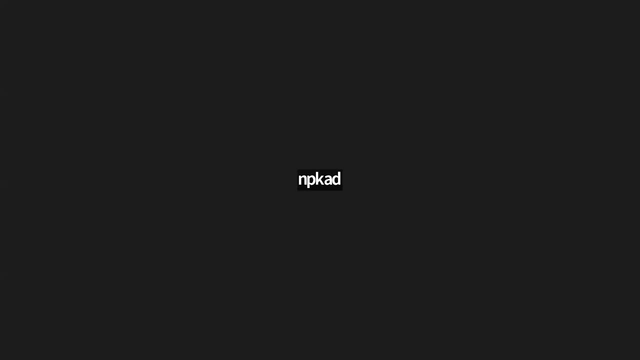 systems and components and get to the same place, And to me it seems like the decision-making would be far simpler if you use margins instead of reliability as the parameter of decision-making choice. Yeah, interesting concept, Prasad, But I agree. 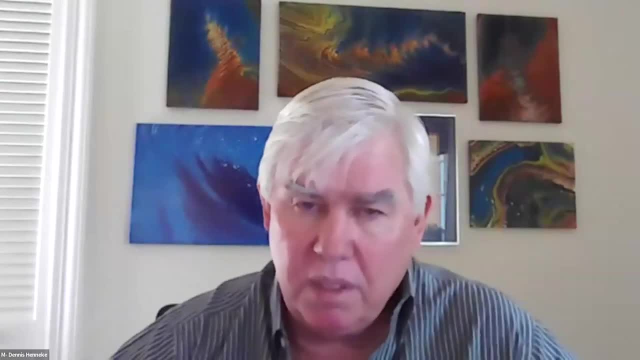 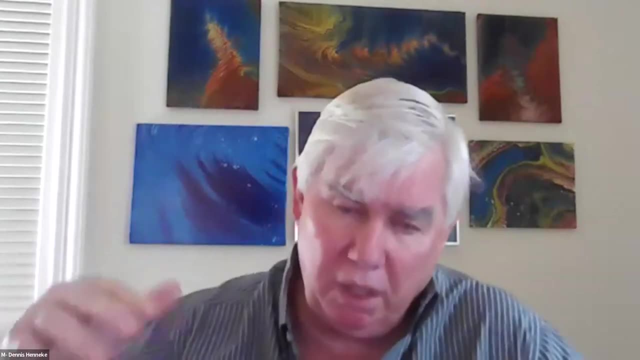 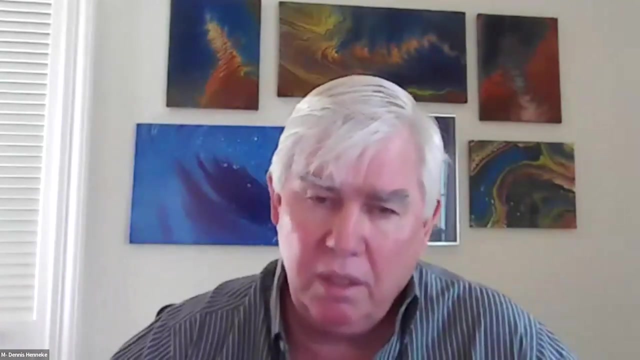 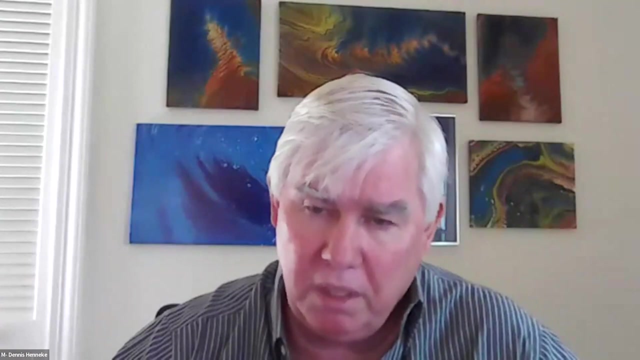 Yeah, Yeah, I would say that the way that the IEA has established performance criteria. there are performance criteria in the lower-level requirements area, such as reliability goals and so on. In one of my earlier slides I said you know the PRA has to be used to establish what the reliability goals are for components, and then you get a performance base. 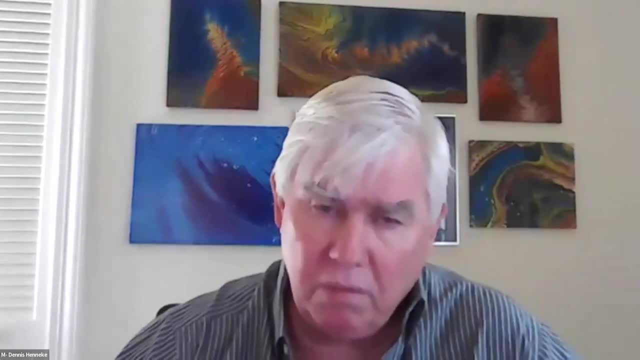 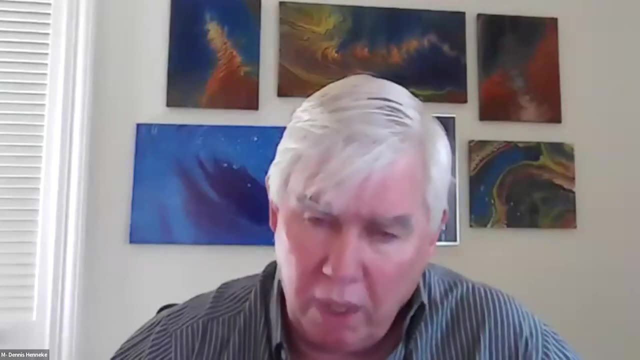 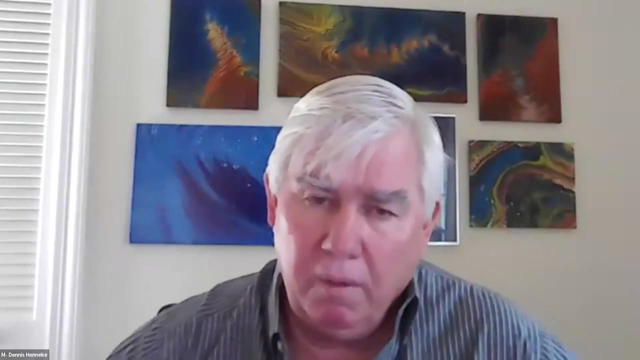 Similar. there's performance criteria under fire protection and other sets of requirements, But in the overall safety strategy the approach you mentioned is not one that would be justified under the current IEA SSR 2-1.. So one could do it that way. 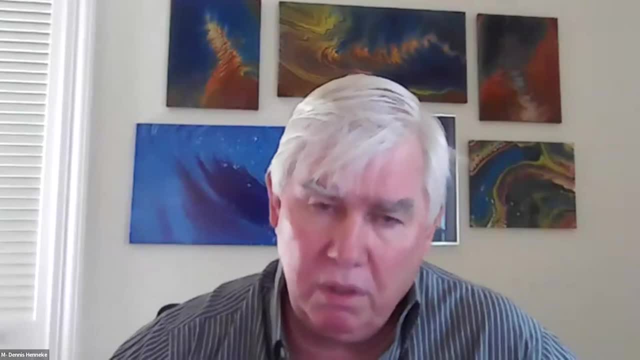 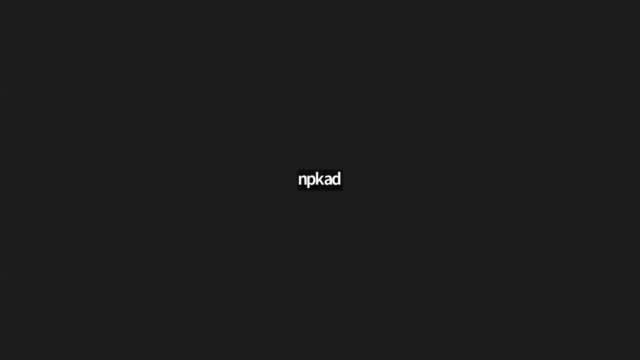 but the SSR 2-1 is not structured that way, So it wouldn't be successful in licensing approach. Again, wouldn't that be country specific? Because in the US we do recognize the validity of the performance-based approach and margins would be completely acceptable. 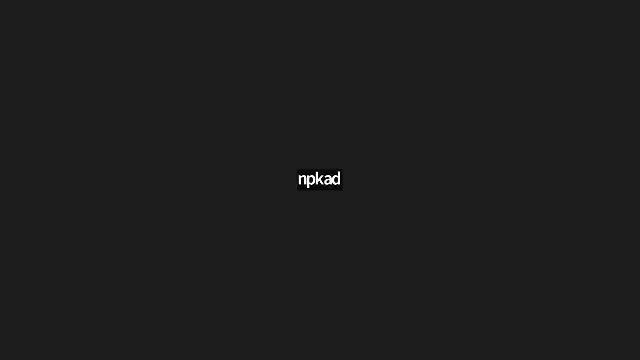 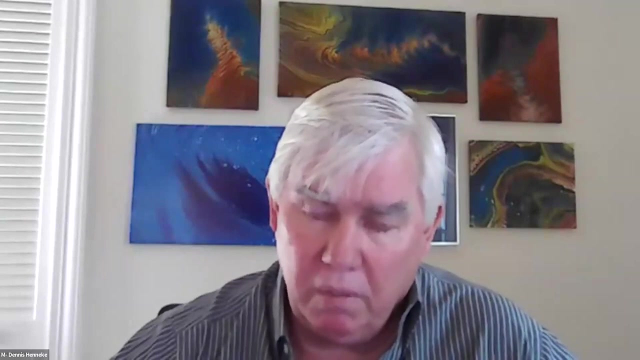 given the commission directions to the staff on risk-informed and performance-based applications. If you're applying SSR 2-1, it would not be country specific. You would meet those And this margins approach, let's say seismic margins and so on. 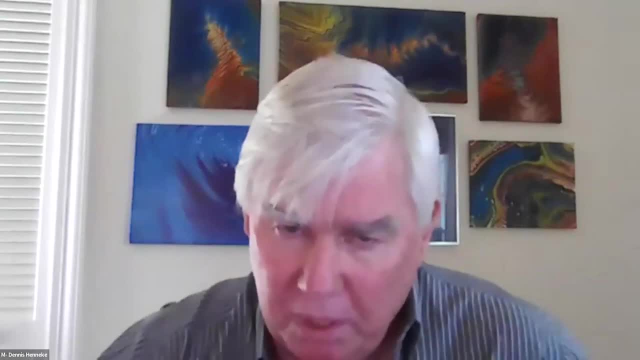 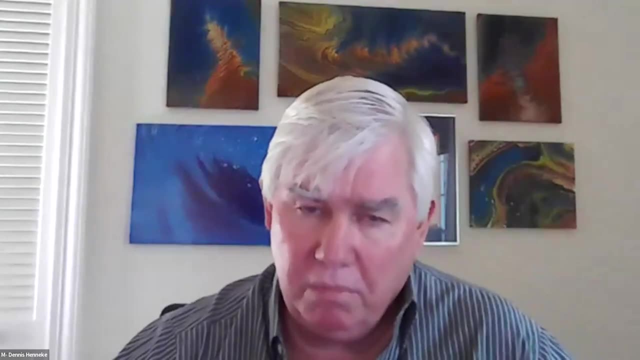 whether you would call that risk-informed or whether you call that performance-based. it's a matter of semantics, because risk-informed and performance-based have a lot of overlap between each of them. So those of us who are risk assessment engineers would call that. 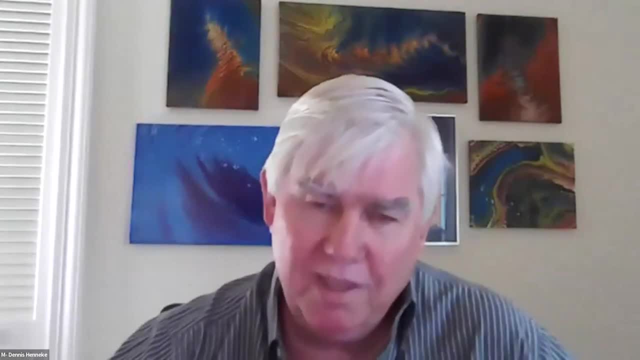 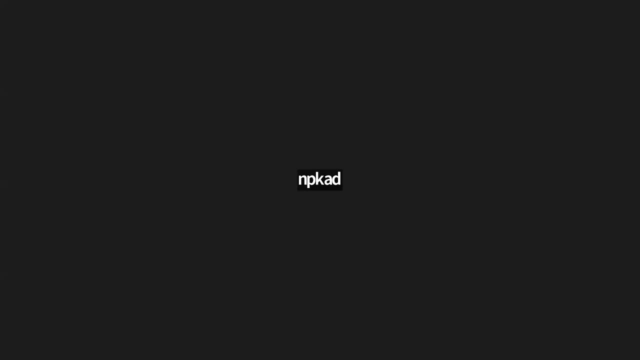 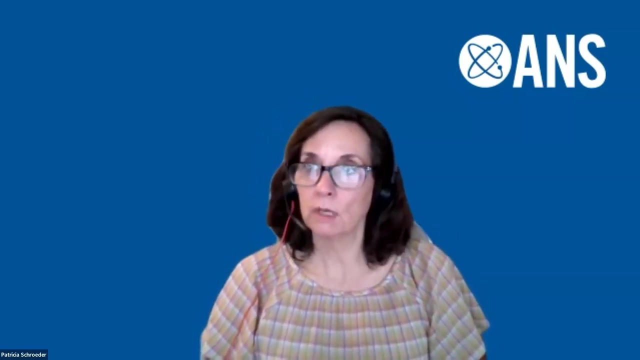 even the margins assessment for seismic, a risk-informed approach, But again, a matter of semantics, I think. Okay, Thank you, Dennis. Thanks a lot for everything. Well, we have one more minute and I don't think we have any more comments. 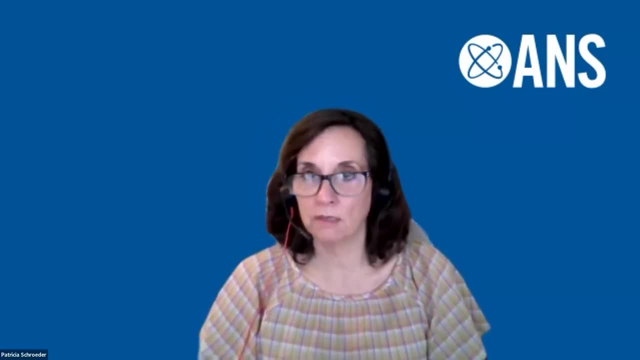 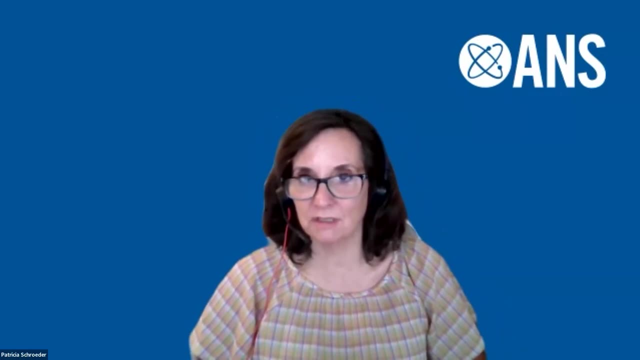 Kent did have to log off. He wanted to make sure that I thanked Dennis on behalf of him and RP3C for this presentation. Looks as if we are ready to close this, So I also want to thank you, And this presentation will be up on RP3C. 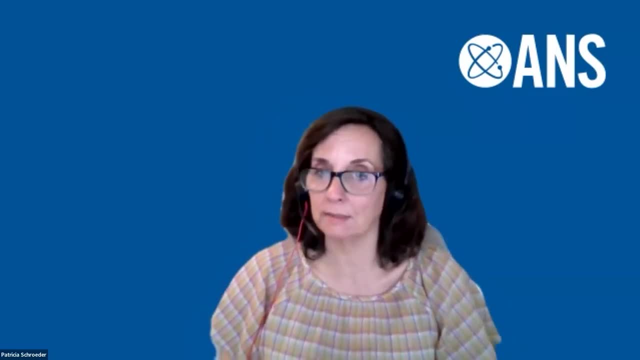 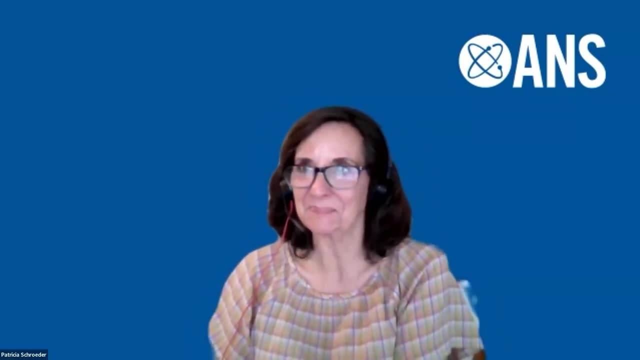 It's a community of practice website, possibly later today, if not later today tomorrow. Thank you all very much. Have a great weekend Bye. Thanks, Beth. Thank you.